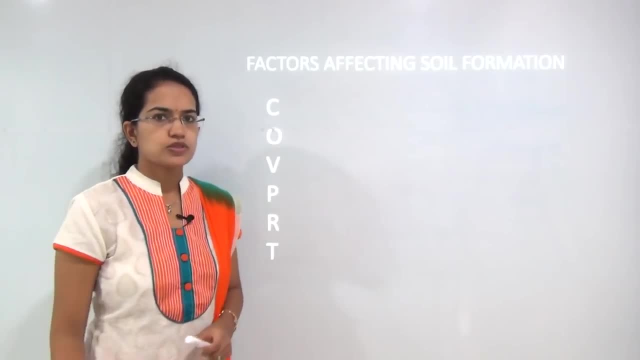 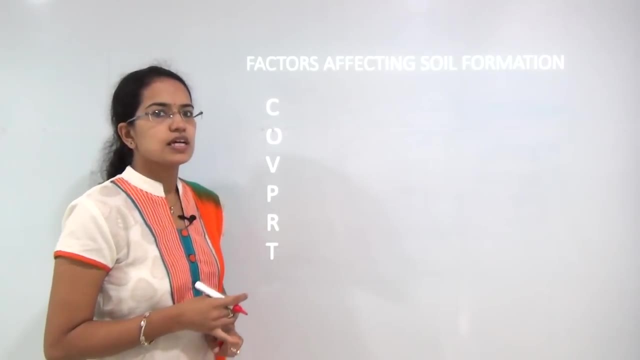 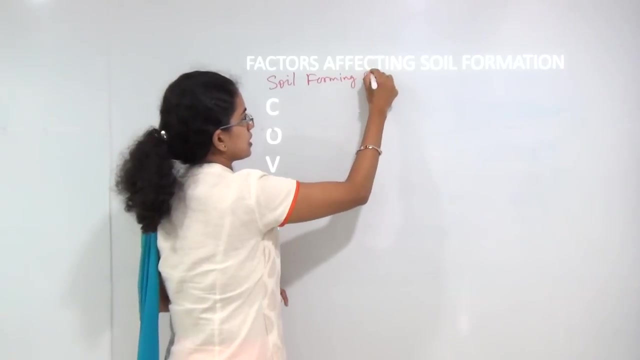 Welcome to this session. In the previous session, we have already talked about soil erosion and the methods of soil conservation. Today, we would be talking about the various factors that affect soil formation and the soil forming processes. So the first thing that we would be discussing today is the factors that affect soil formation. 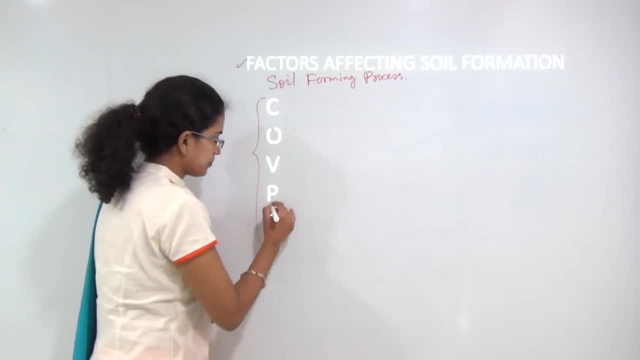 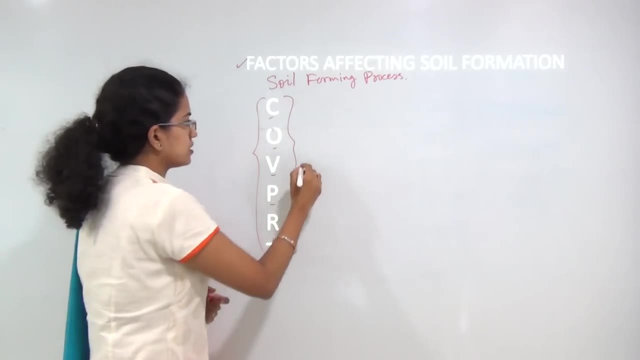 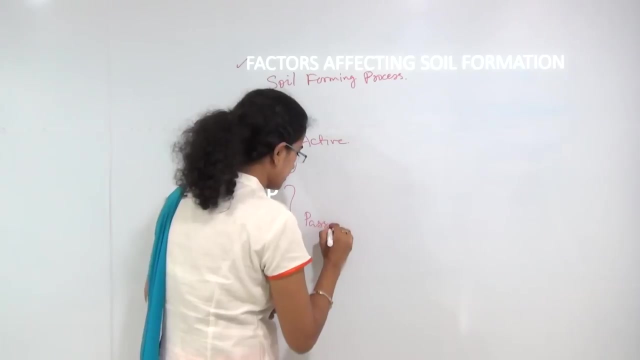 Now you might be surprised as to what does this code word mean. So that is a way you can remember the factors that affect soil formation. The first three factors that I have taken into account are considered as active factors, and the last three factors are passive factors. Now let us first discuss the active factors. The first is the climate. 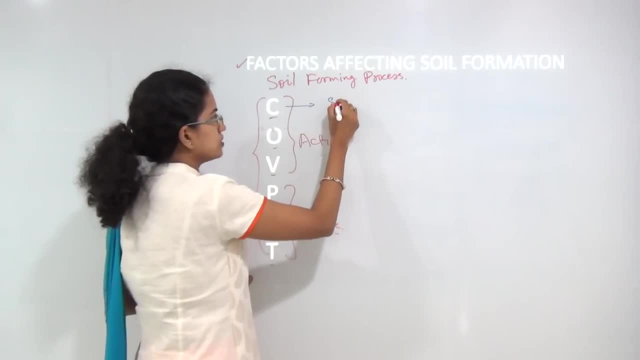 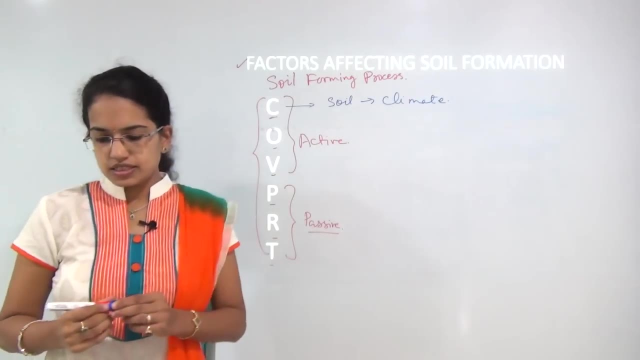 the climate of any region affects the type of the soil. So soil is affected by climatic conditions. So if there is a kind of a soil formation, the climate of any region affect the type of the soil. So that is size, the soil formation. so if there is a kind of soil formation, that 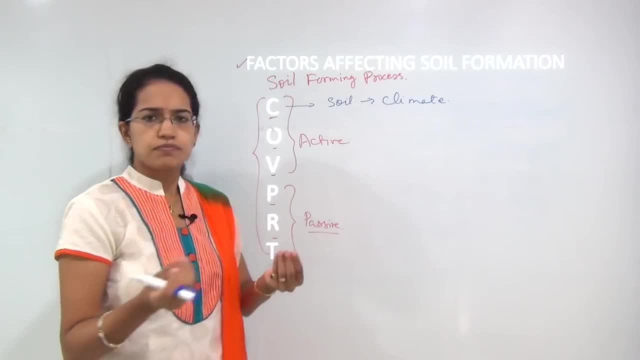 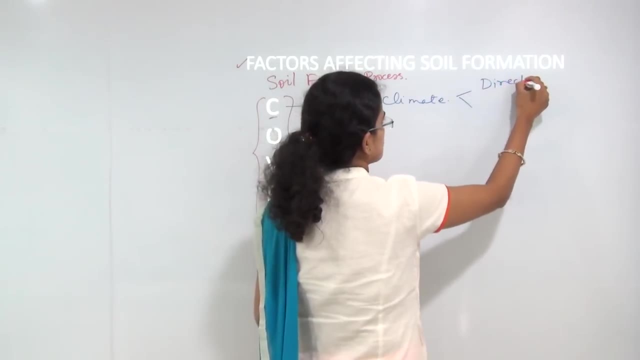 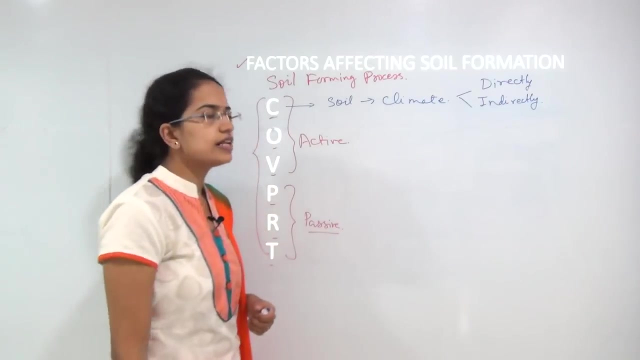 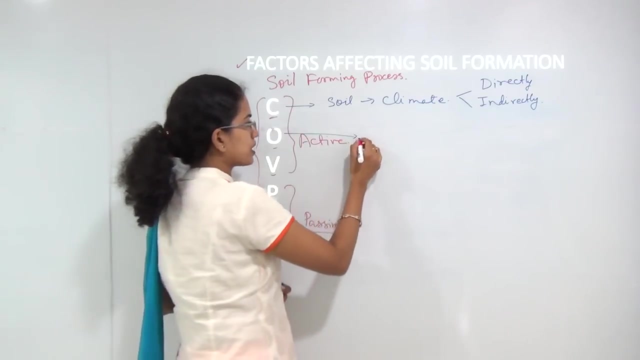 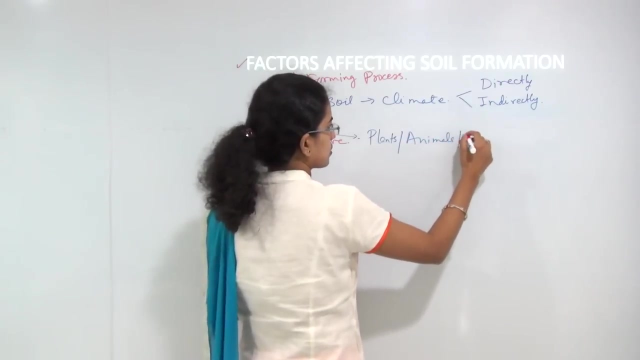 of very dry weather, the soil would be desert soil. climate directly and indirectly affects the soil. if I say directly, I mean by means of rain or wind. if I say indirectly, it can be by the flora and the fauna that exist in the region. The next is the organisms. it includes plants, animals and other microorganisms. 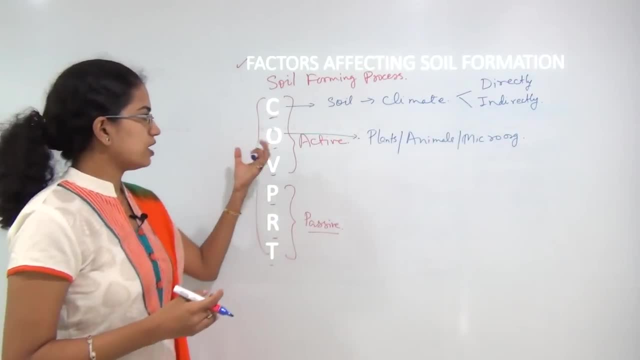 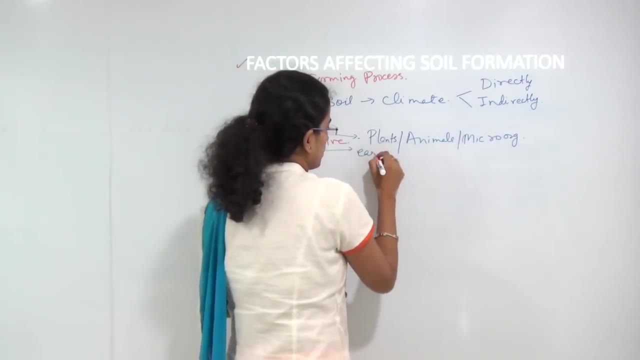 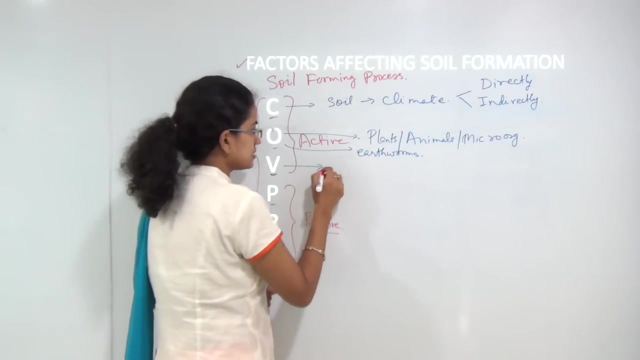 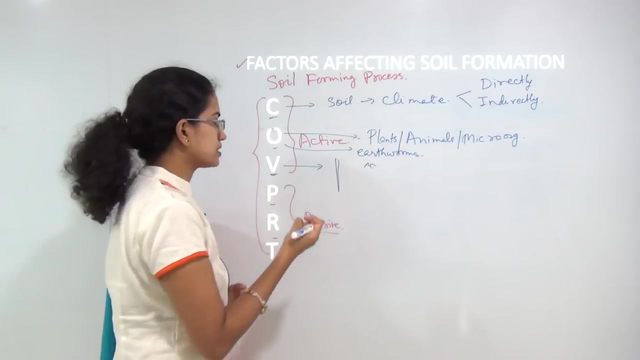 So when we talk about plants, animals, microorganisms, they all affect the activity, the formation of the soil. for example, if you have lot of earthworms in the soil, the soil will become porous. The next is the vegetation, As we have already talked about the root system, some roots hold the soil very firmly as compared. 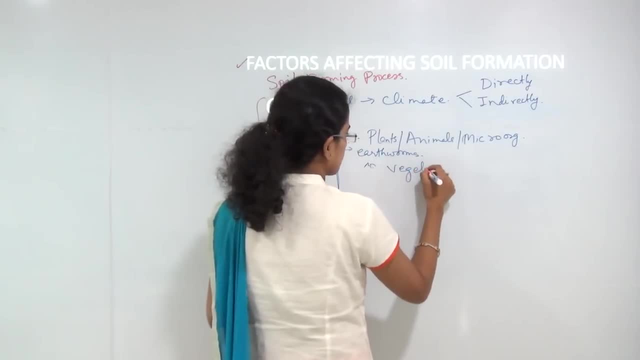 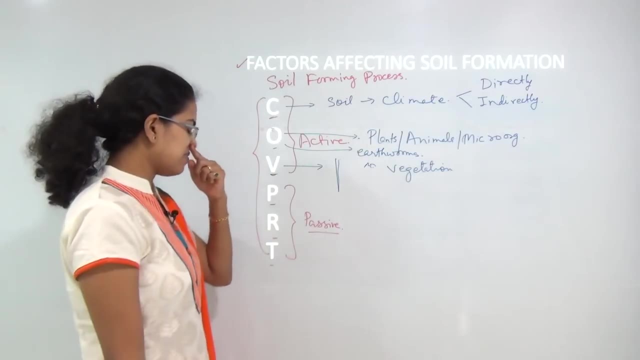 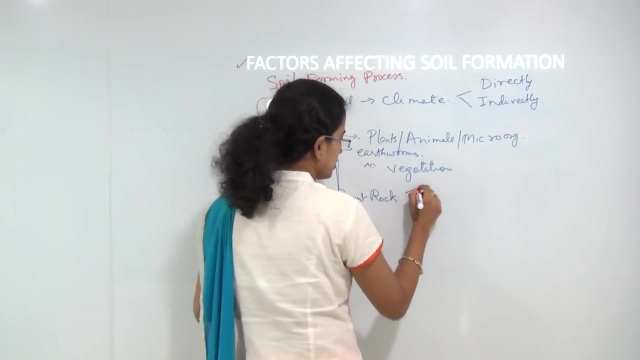 to other roots. so vegetation is another important criteria that affects the soil formation. Now let us go on to the passive factors. The first passive factor is the P, that is, parent rock. Now, parent rock can either be sedentary- Sedentary means. 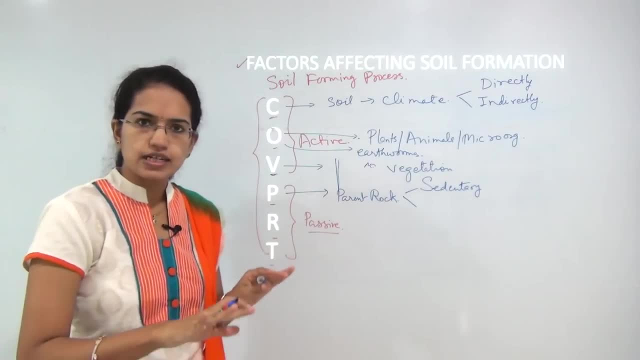 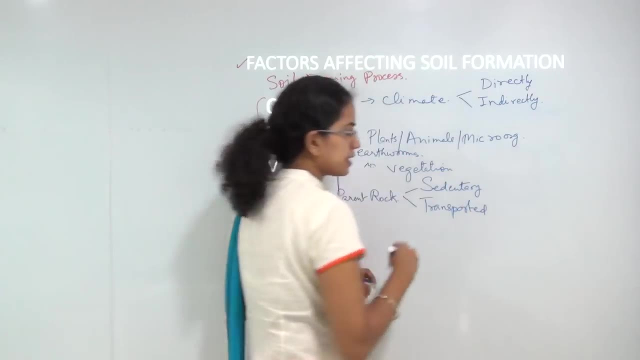 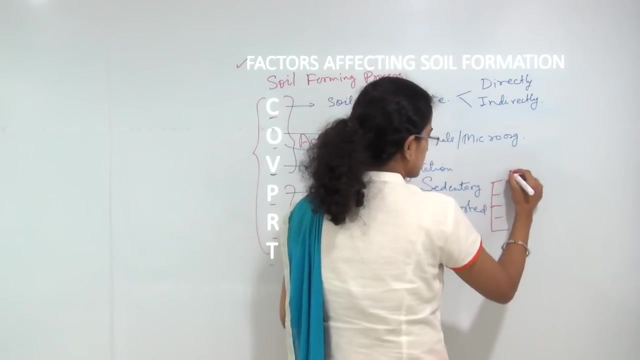 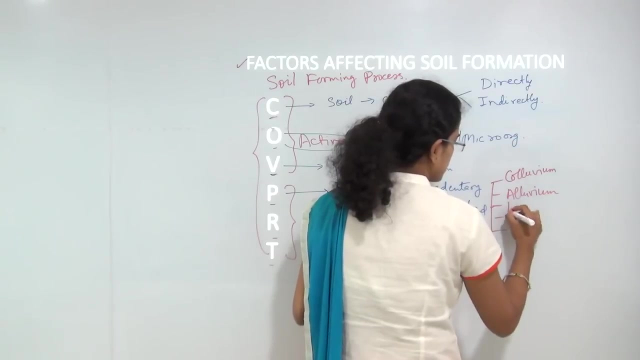 It is fixed at, it is located at a particular position and the next is transported. Transported means it can move from one place to another. Now, transportation can be of various types. I can have n number of explanations. first is collovium alluvium lochestrine. 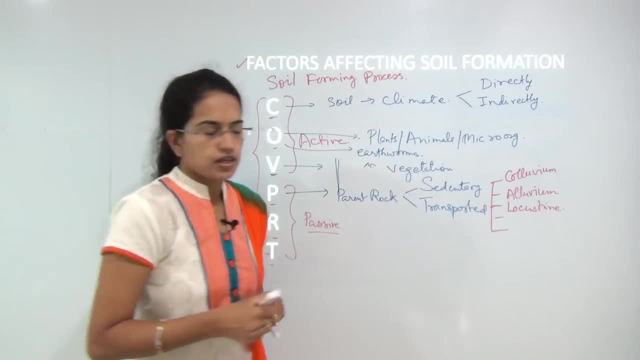 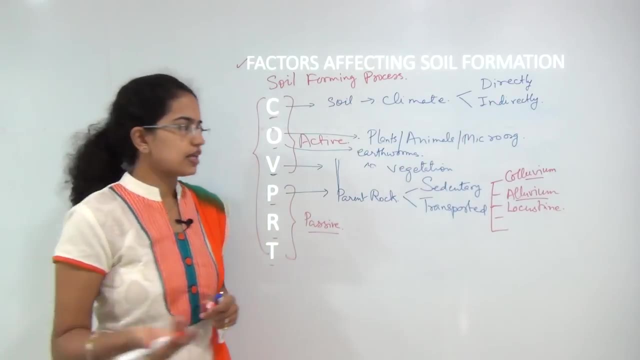 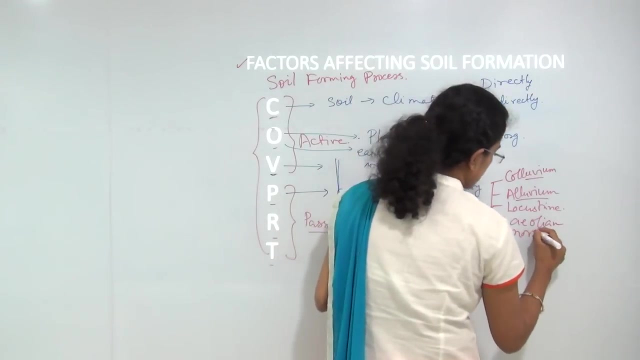 So what is lochestrine means Near the lakes? Collovium means due to glaciation. alluvium means due to movement of water particles. Then you have aeolian that is due to wind. You can have moraines that are glacier remains. 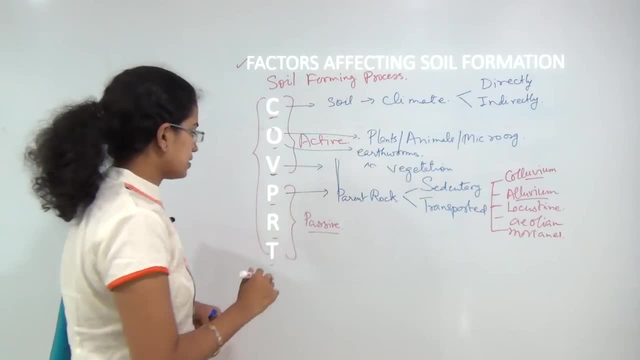 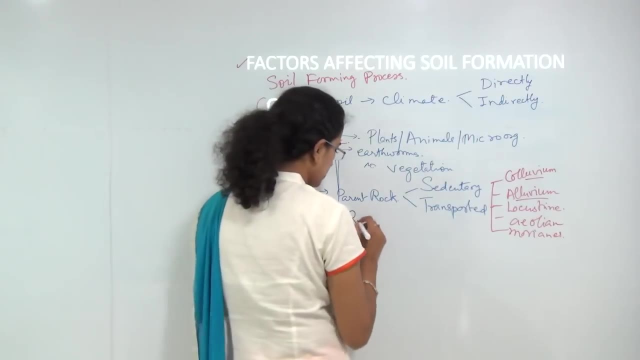 So there can be various types of transportation material that can take part. The next is R. R means the relief, The relief of the region, The relief of the region. R is another kind of surface Can vary from, say, flat areas with 0 to 5% of slope. 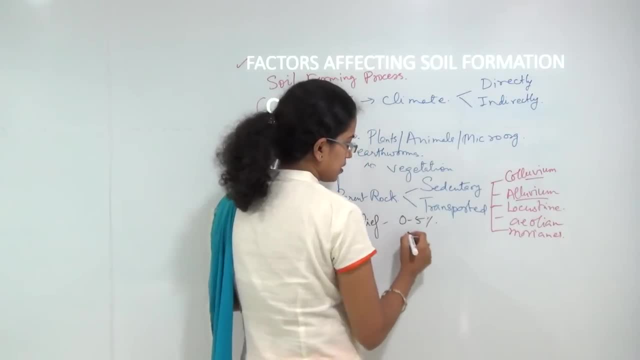 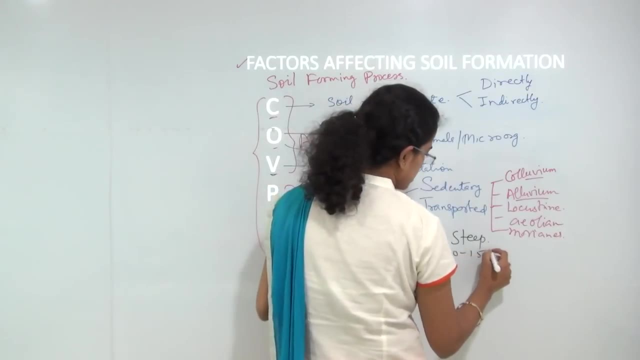 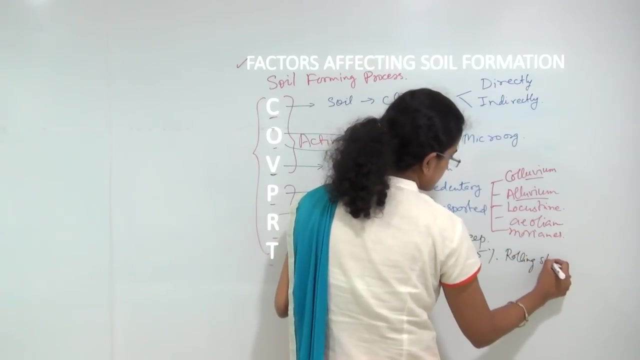 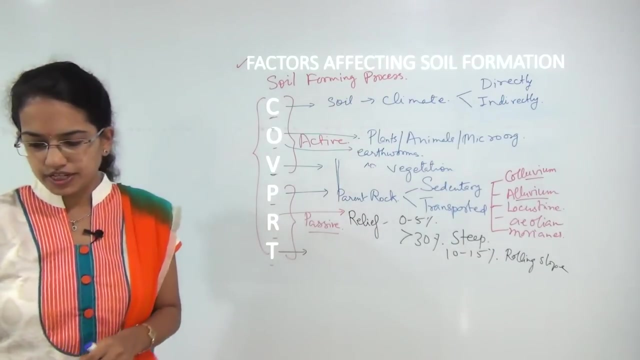 A slope of greater than 30 is considered as steep slope. Then around 10 to 15 degrees percent of the slope, I would say it is a kind of a rolling hill or rolling slope, So the relief also makes a soil formation. And last is T, which stands for time. 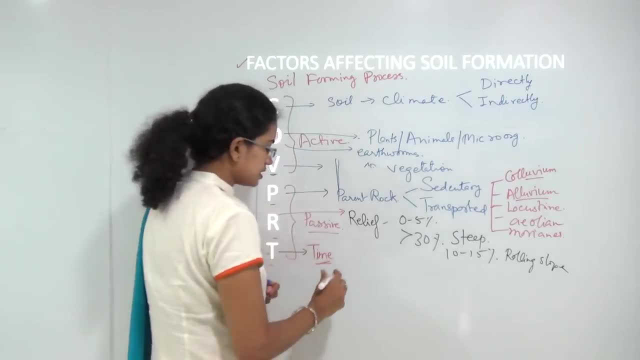 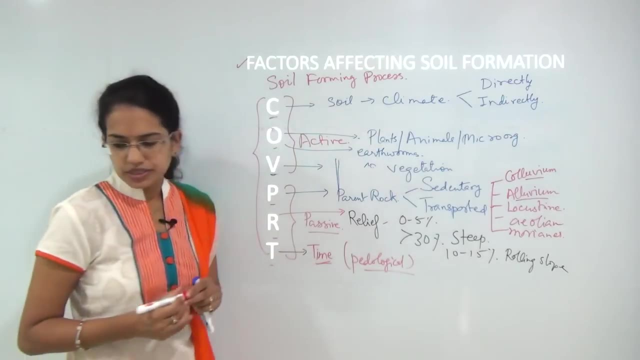 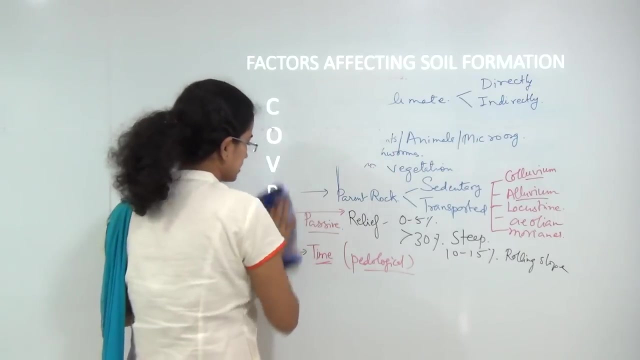 Usually, in case of Time Soil, we also call it as pedological time, and that denotes the time that is taken for the formation of the soil structure, and usually it is considered in thousands of years. So these were the basic factors that affect the soil formation. 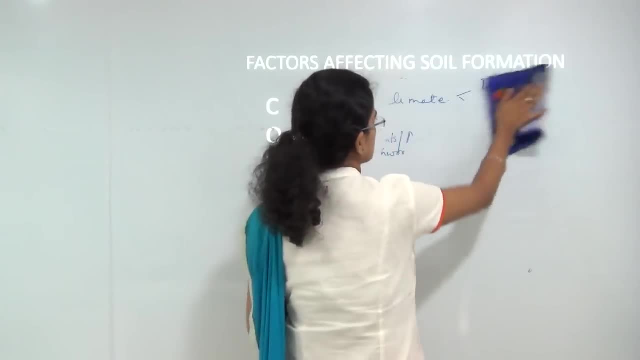 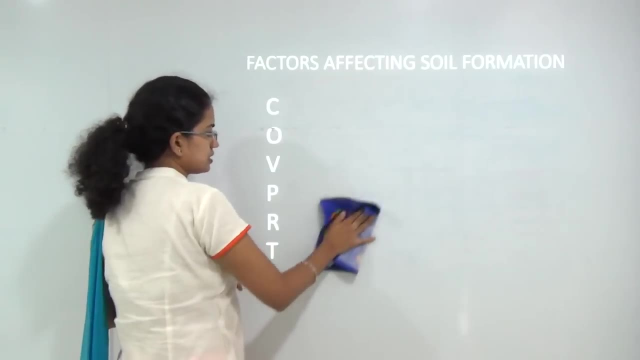 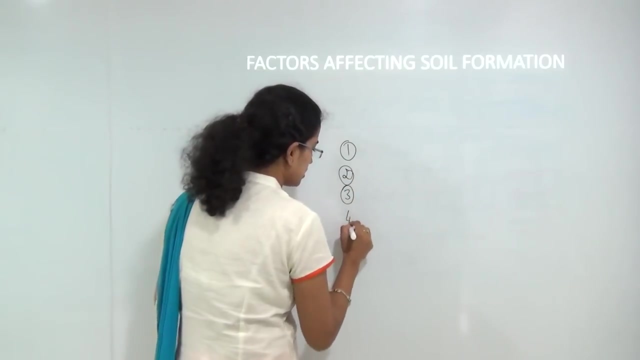 Now let us understand the processes. When I talk about processes, I broadly classify the processes into 4 types. The first is addition, the next is losses, the third is translocation and the fourth is transformation. So these are the 4 processes I usually talk about. 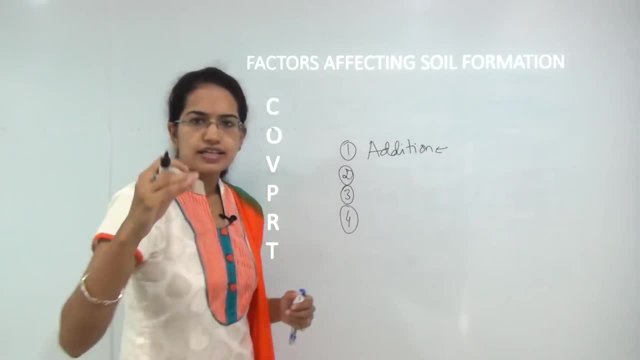 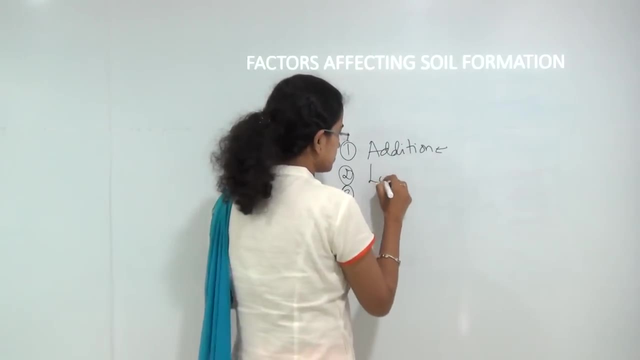 That is addition. that is addition of either leaves, humus or any kind of layer of sand. that would be addition. Losses can be due to various factors. they can be due to erosion, they can be due to weathering, They can be due to leaching. then is translocation and transformation. 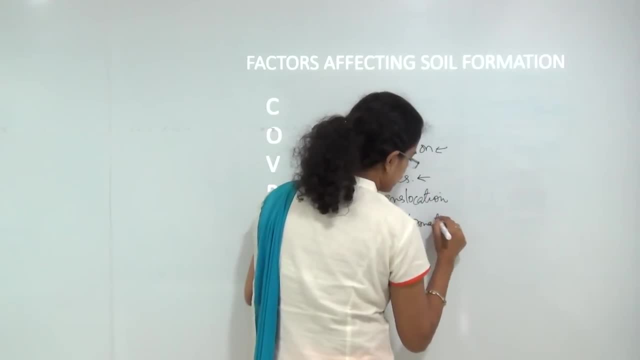 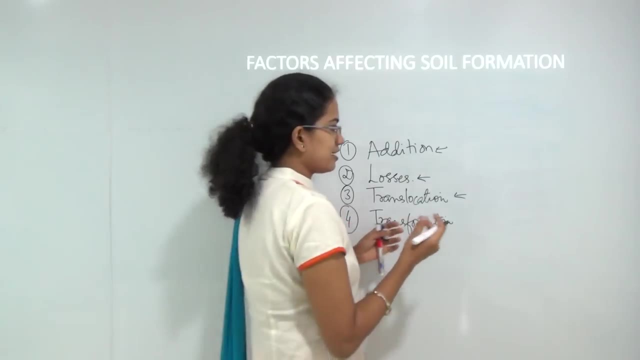 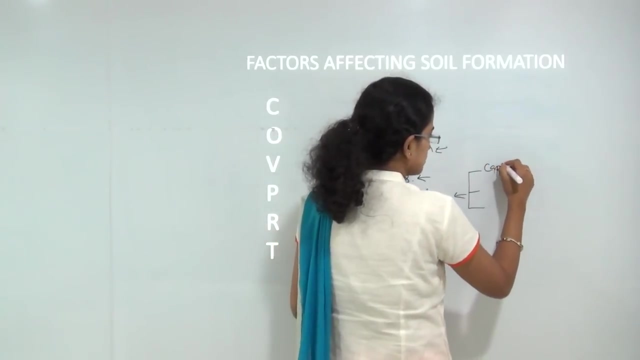 Now let us understand the difference between translocation and transformation. Translocation is movement from one part to another. So translocation involves kind of capillary action leaching process. So under translocation we would be talking about capillary action. I can say translocation. 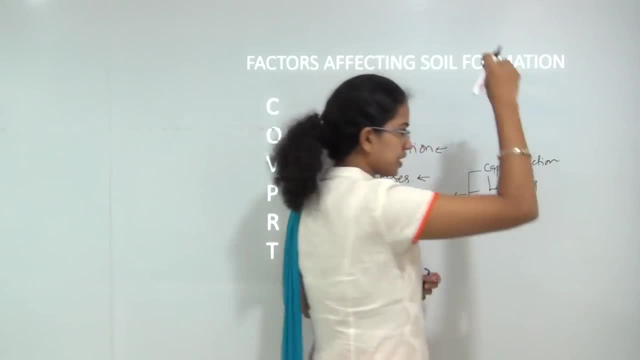 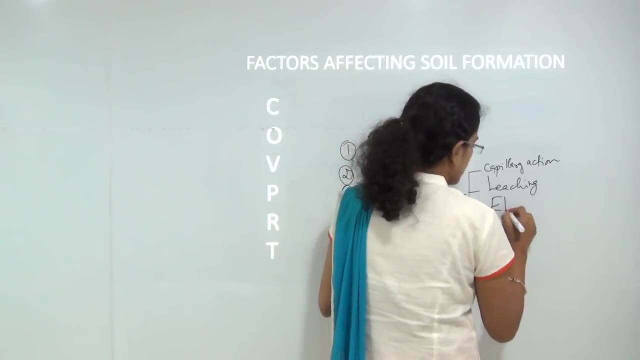 Translocation includes leaching. So, due to rain water, what comes down? the top layer of the soil gets off or the humus get removed. Then you have eluviation that is removal from the top layers, and eluviation that is deposition. 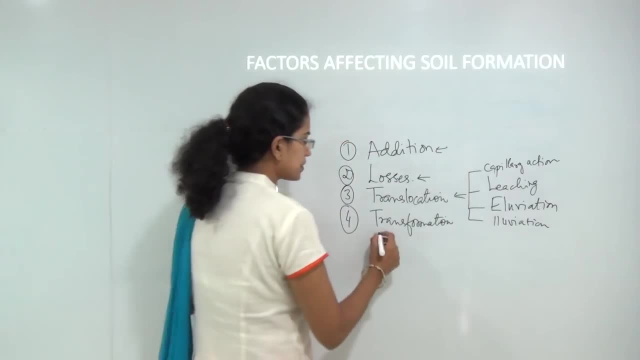 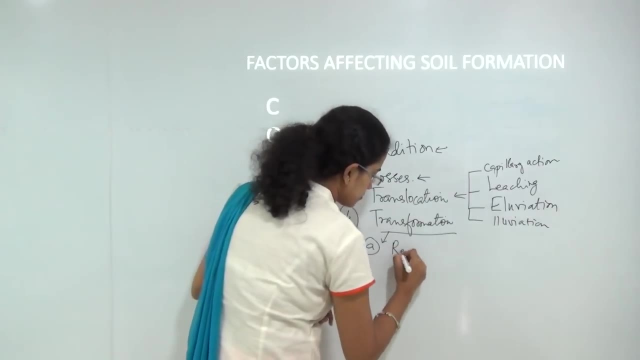 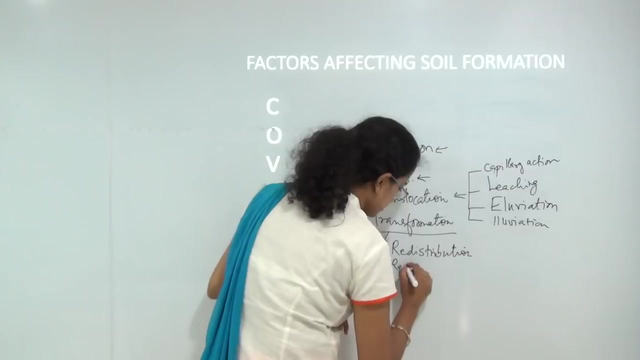 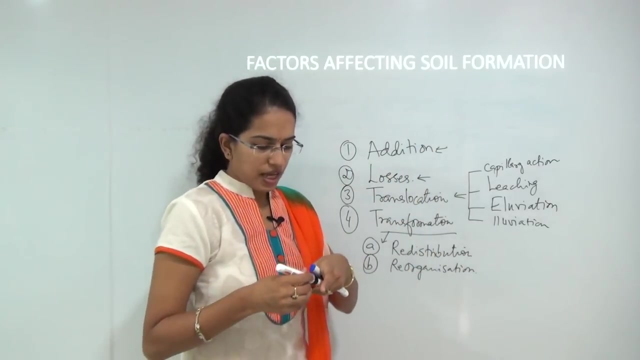 into the lower layers. Then you have transformation Under transformation. we would discuss about 2 specific things, That is, a- Redistribution, Redistribution And b- Reorganization. So redistribution means distributing the same particles again And reorganization means either I am changing the shape of the particle or kind of changing. 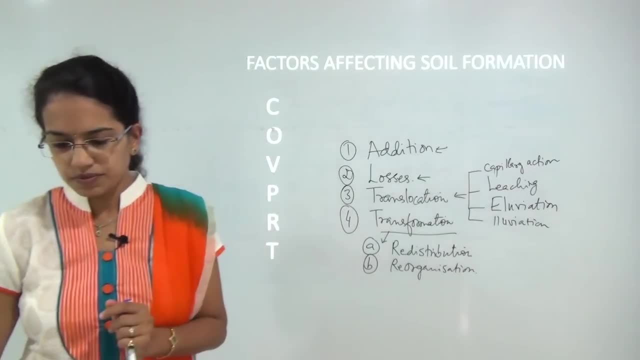 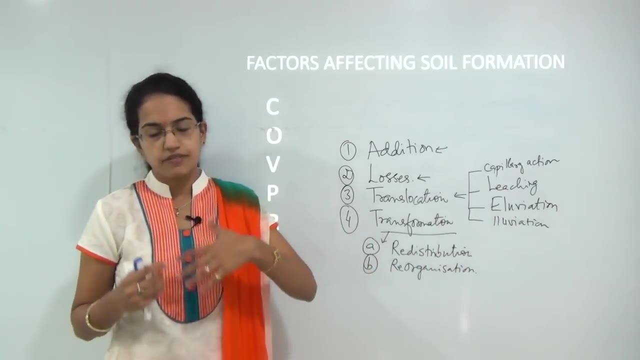 the process of arrangement of the soil particles. So transformation can be either through redistribution or reorganization. There are various processes involved in transformation. The first process is de-organization. The second process is inter-organization. The third process is inter-organization. 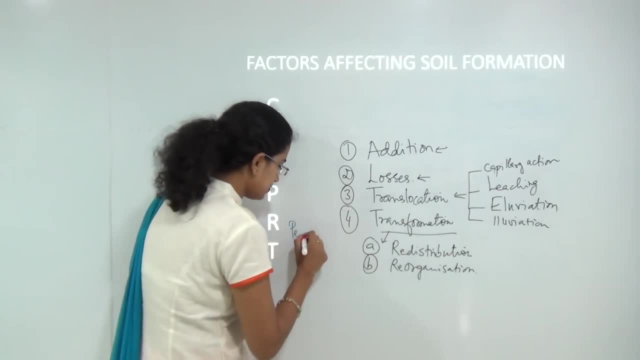 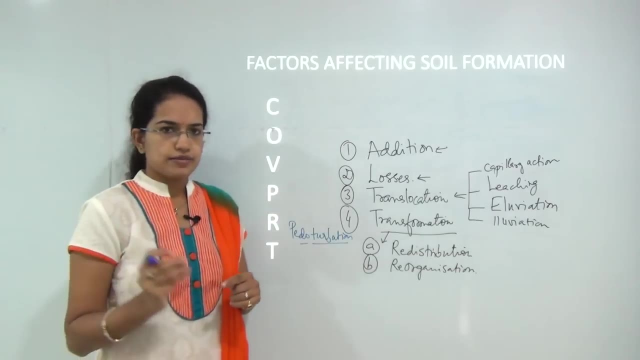 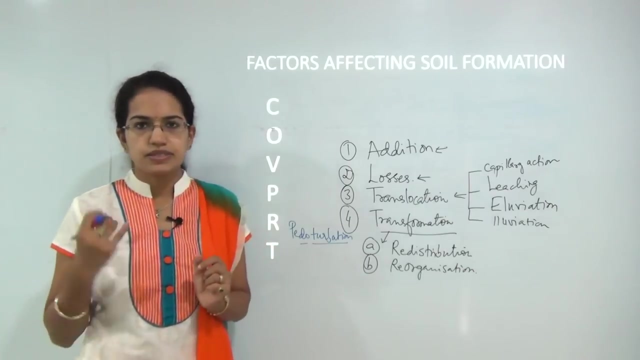 The first and the foremost is pedotervation. that is due to small animals. when they, along with them, they move the particles of sand or soil. that is known as pedotervation. Besides this, there can be humification, there can be compaction and there can be other processes. 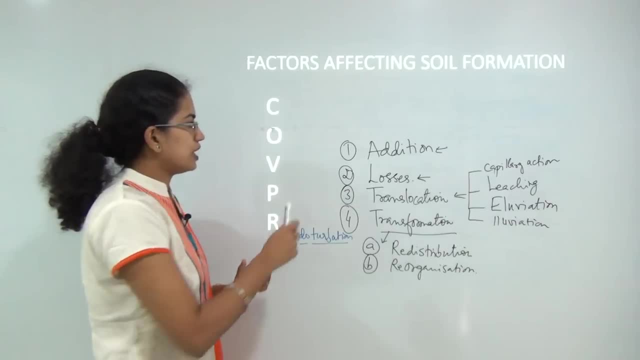 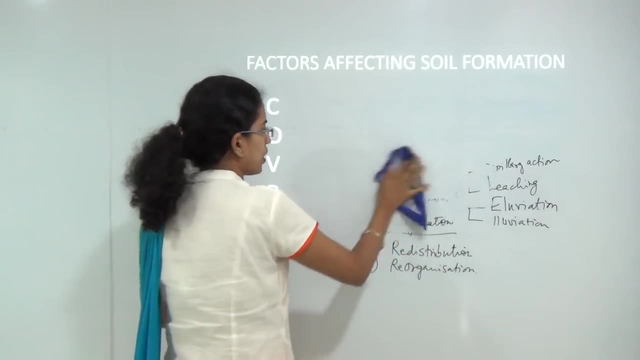 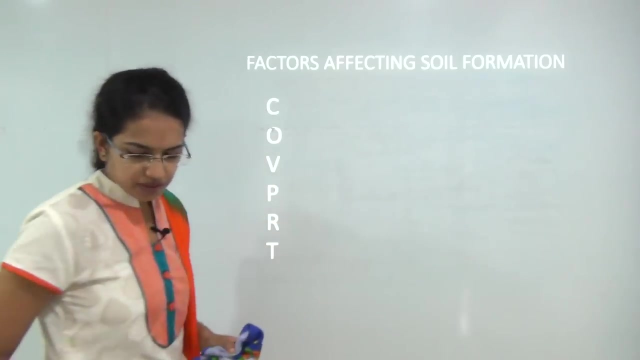 and transformation, which we would be discussing further. So let us first talk about addition. that is the first process. So, as I said, leaves, humus, particles, humus or addition of other layers of the soil would be considered under addition. So I have the first process here. 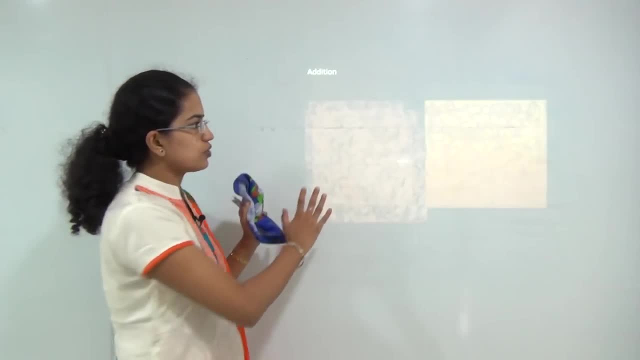 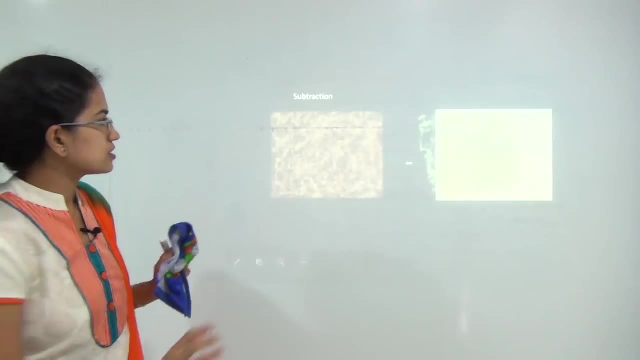 So you have the addition of the soil on to the existing soil, as you can see. So that is the process of addition. The next is losses. So you are, the top layer is being removed from This soil, So this soil is suffering a kind of loss. 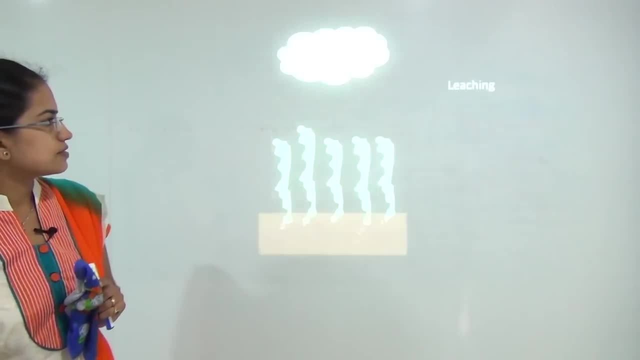 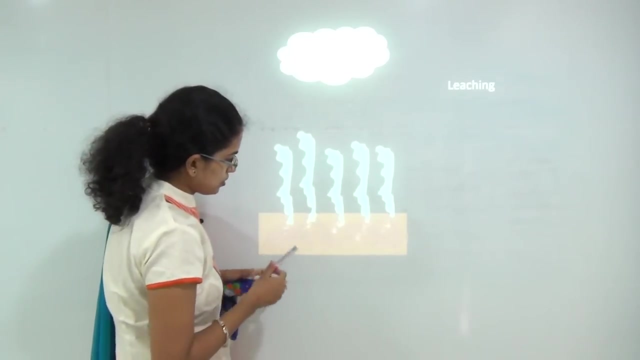 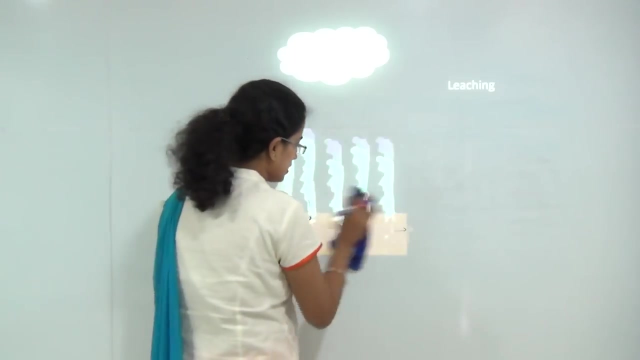 So it is a kind of losses. The next is leaching, So as the rain water falls, you have the soil layer that is moving out, So you have rain water coming down and you have soil that is moving away, So the top layer is being washed away. 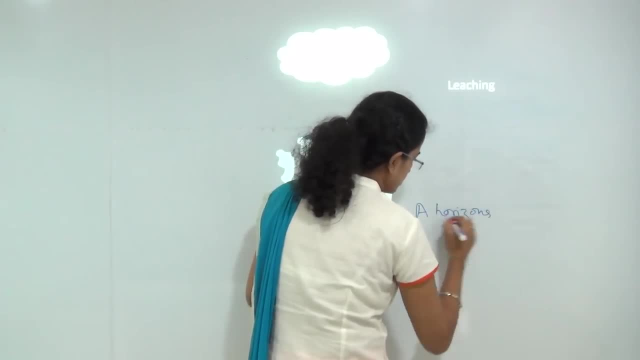 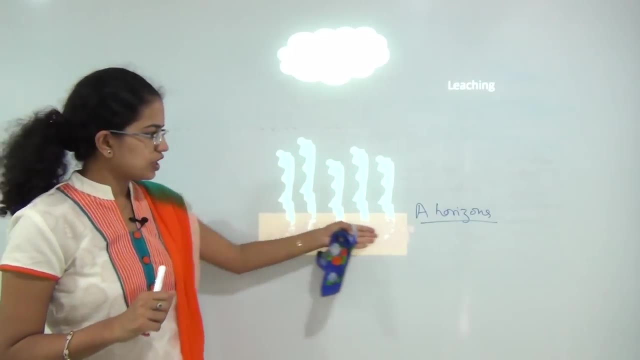 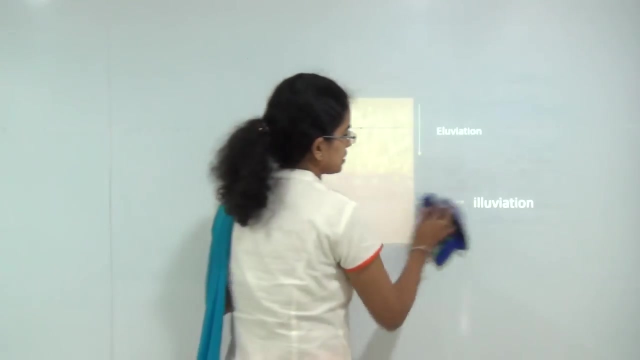 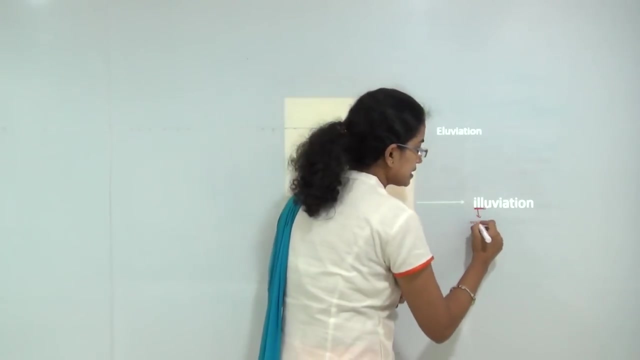 Usually occurs in A horizons. So let us talk briefly about what is leaching. So leaching occurs in the top layers, removes the humus and occurs due to rain water. The next here is eluviation and eluviation. So when it is IL, so I, where it stands for I can say it is in. 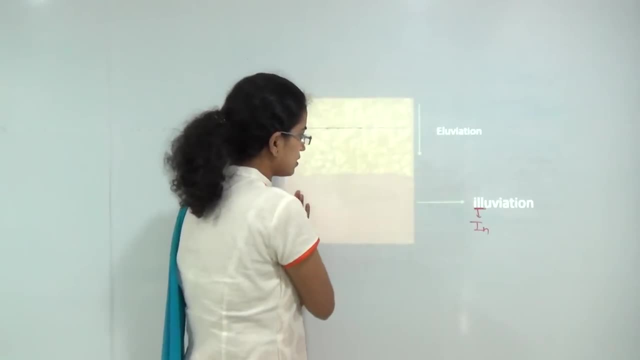 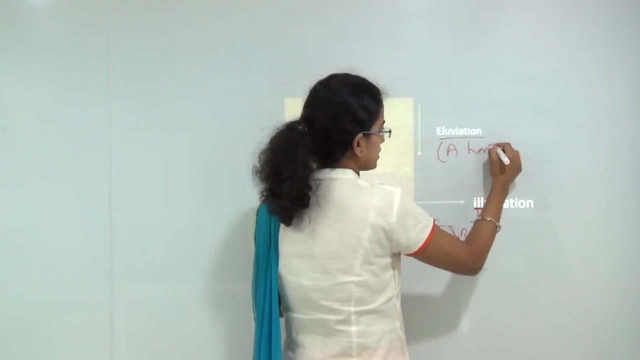 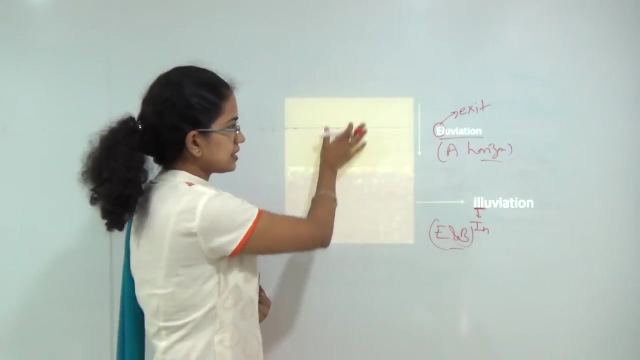 So it is accepting the things, So it is. eluviation is accepting the deposits common in E and B layers. eluviation common usually in A horizon, So under eluviation is exit, E for exit. So the sand is exiting from here or the soil particles are exiting from here and getting. 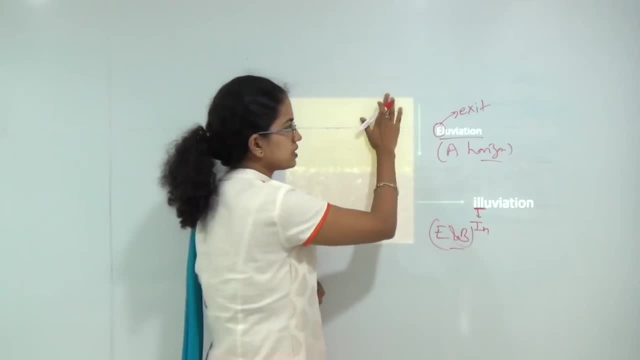 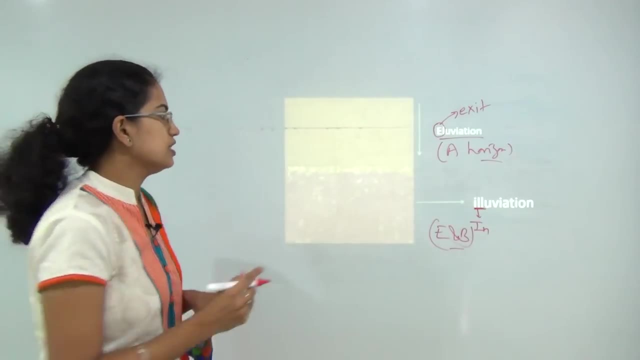 deposited into the eluviation zone. So eluviation is the area of removal, eluviation is the area of deposition in the broad sense, if I try to understand. So both these processes fall under translocation. Then you have next which is known as transformation. 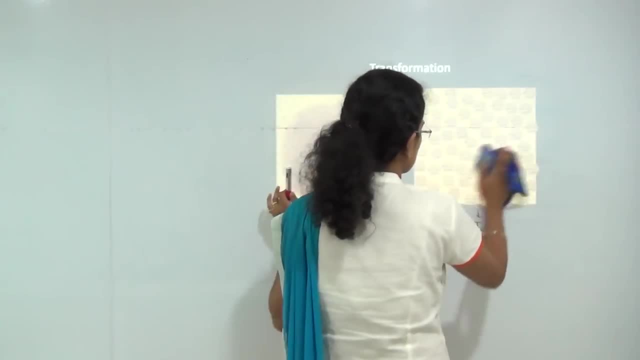 So transformation, as I said, is reallocation. So transformation, as I said, is reallocation. So transformation is reallocation. So you have original sand particle which is of this shape. It might get reorganized as hexagonal or circular form, So it is changing. the form is what is transformation? 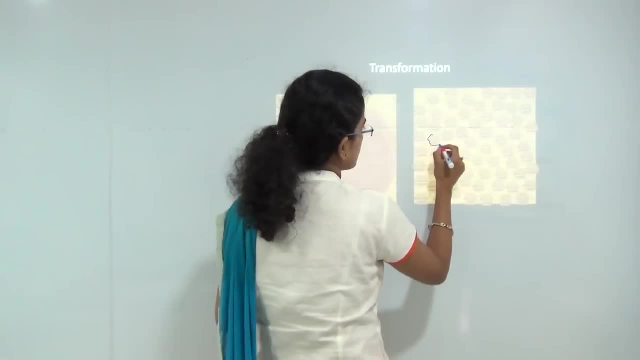 Now there are few terms that we try to understand under transformation. The first is humification. So what is humification means? I am transforming the raw material that I have into humus. that is what is known as humification. So what is humification means? 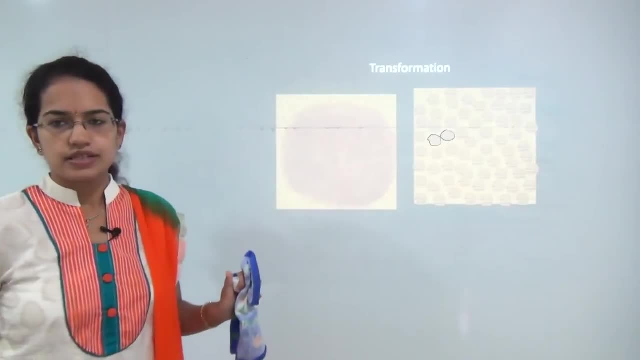 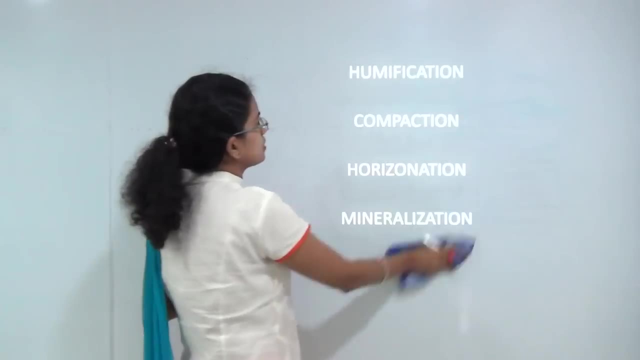 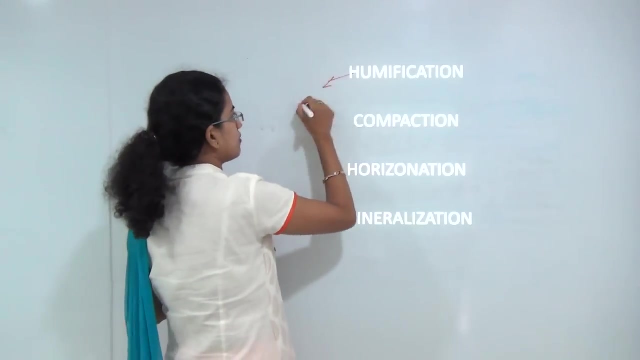 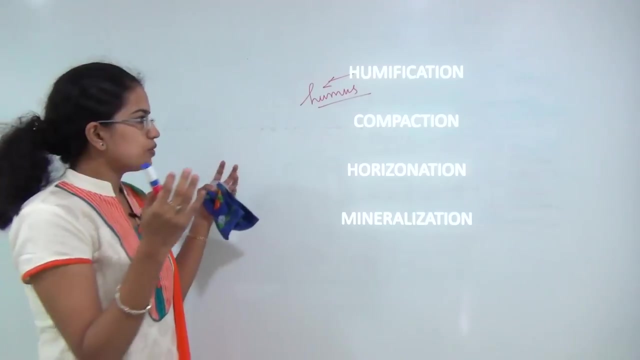 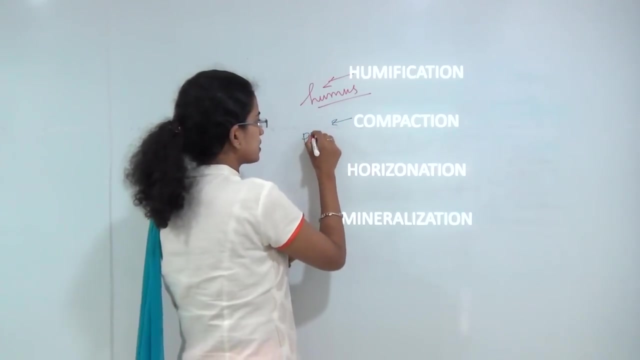 I am transforming the raw material that I have into humus. that is what is known as humification. The next is compaction. due to compaction, the soil is getting closer, and when it is getting closer, percolation becomes difficult. So that is what is compaction. 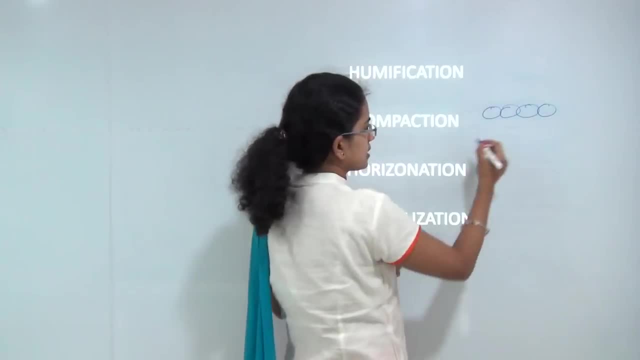 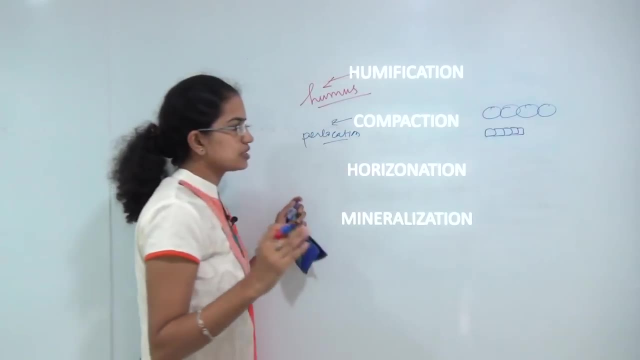 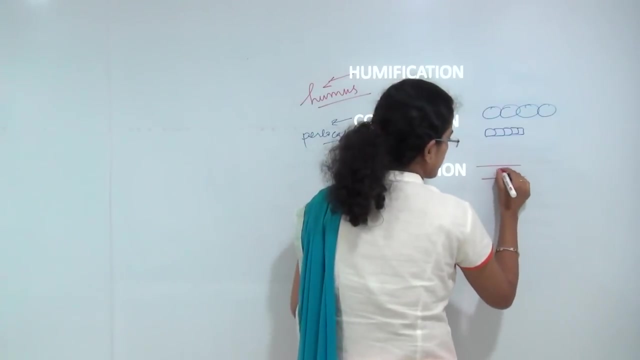 So I have initial soil particles which are, say, like this, and I have the next soil particles which get tightly packed. So that is what is compaction. Horizontation means I have soil differentiation in various horizons. So I have A horizon, I have A1, A2, A3.. 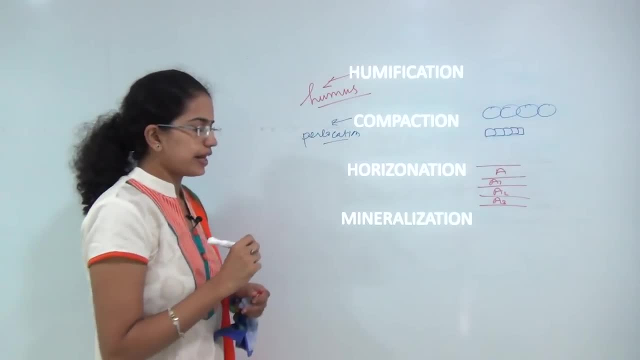 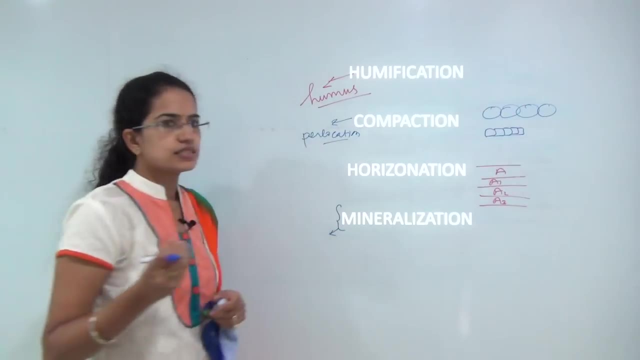 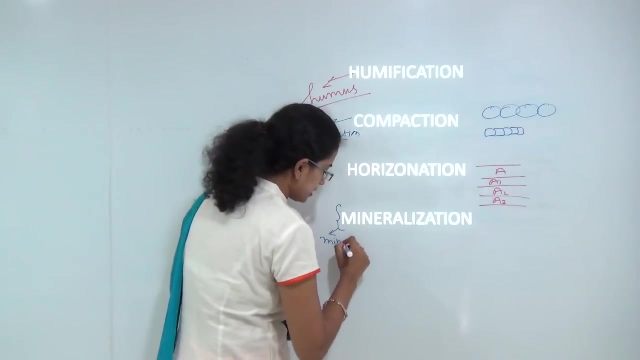 So I am getting differentiating the soil into various horizons. And last is mineralization, where the chemical composition is being changed. I can say there is removal of ammonia or there is kind of mineral change or chemical change that is taking place in the soil layers. 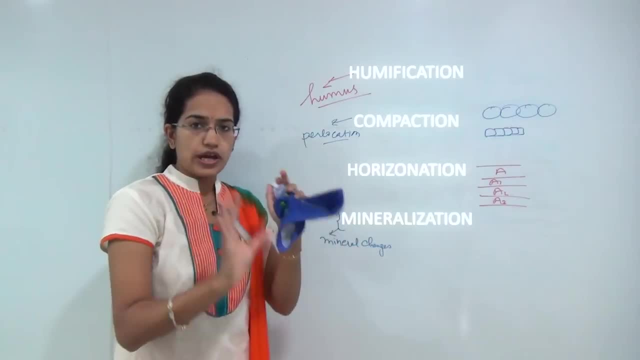 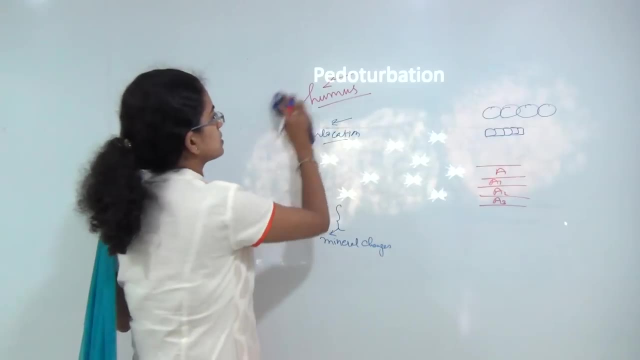 So these are some of the forms of transformation. The soil remains the same, only it is being reorganized or reordered into some other form. And the most interesting is pedotermation. So pedotermation, what happens is there can be animals or small microorganisms. what they 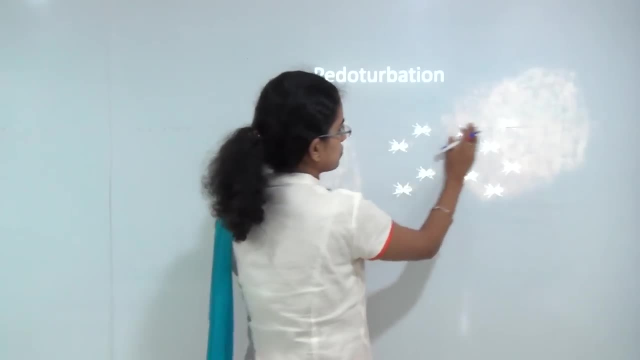 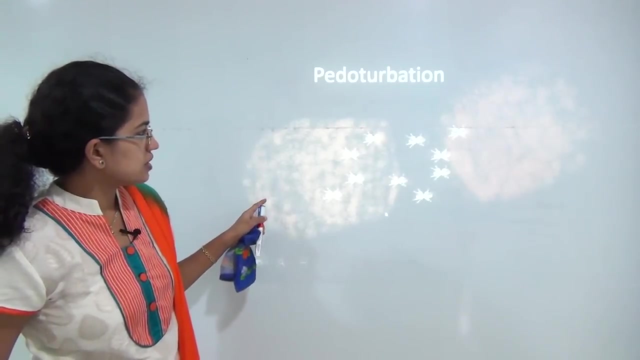 do is they transport the material from one chunk of soil to another chunk of soil along with them. So, as you can see, here you have the particles with what is known as ajaim. What are the particles? you have the organisms which are taking the sand particles along with them, and that is. 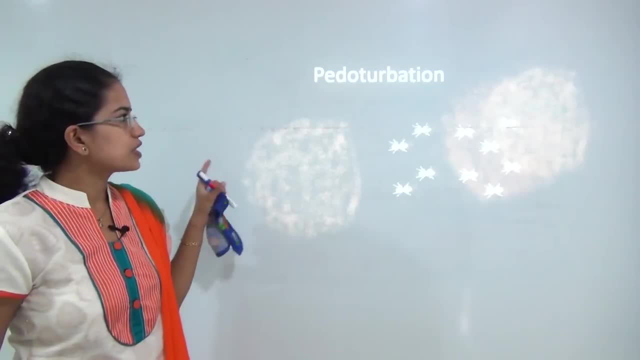 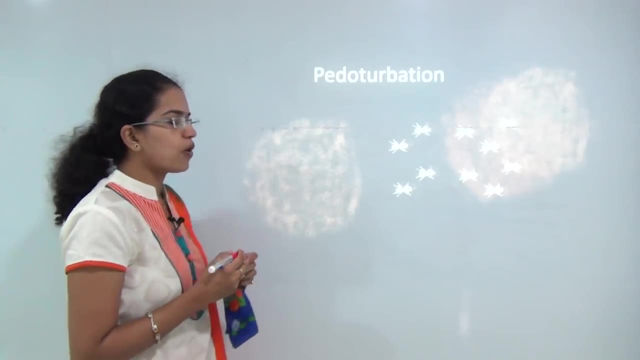 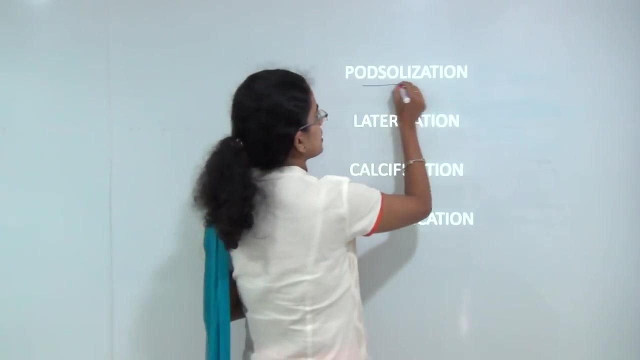 what is explained by pedoturbation. Now, with this we covered the basic 4 processes that help to form the pedoturbation, or the soil processes. Now we will move on to the specific soil processes. The first specific soil process that we would be talking about is podocelization. podocelization- is usually found in coniferous areas or coniferous forest, where the temperature is low. Now what happens under podocelization is the soil becomes acidic or, since the soil is in the low temperature region found in cold, mid humid areas, the soil gets bleached off. 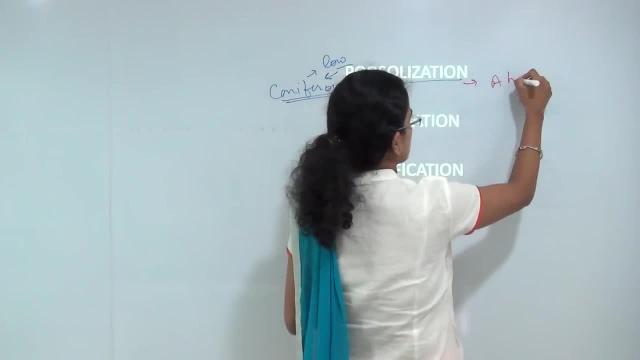 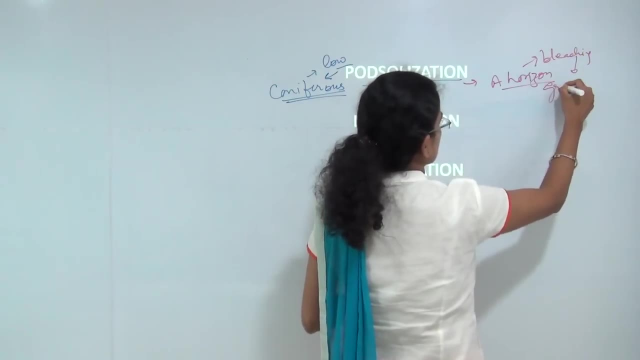 So the uppermost layer, or the top layer, or the A layer of the A horizon of the soil gets bleached off, Okay, And due to bleaching, it becomes either grayish or blackish in color. So that is one of the major implication of podocelization. 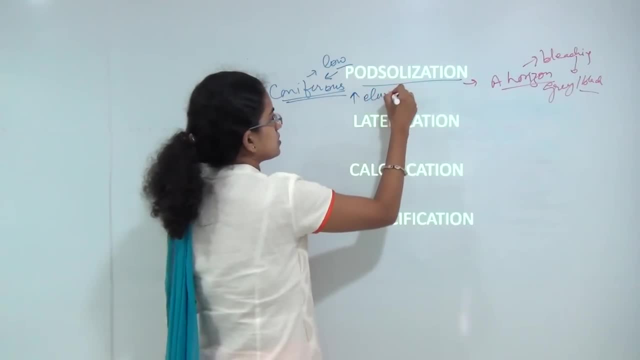 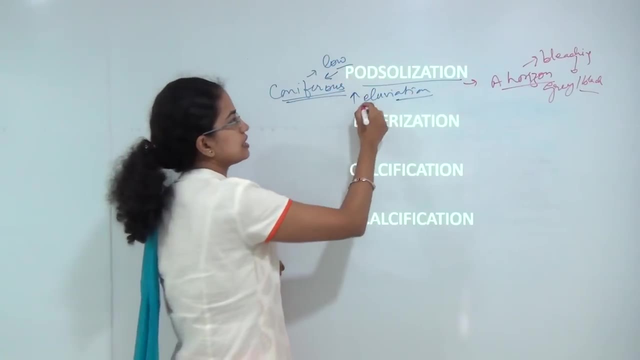 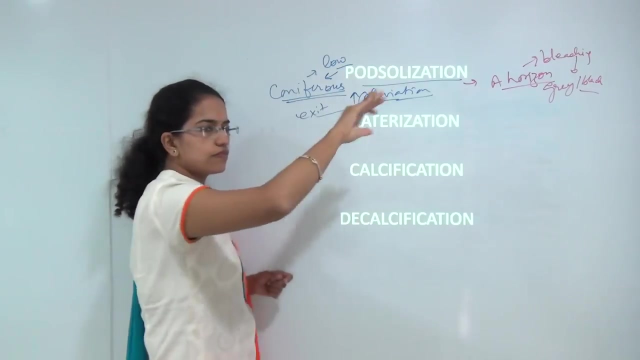 It increases the process of eluviation, since the soil is being drained off of the existing nutrients. it is being removed. So what happens is there is increase in eluviation process. So eluviation, as I said, E stands for exit, so it is removal of the material from the 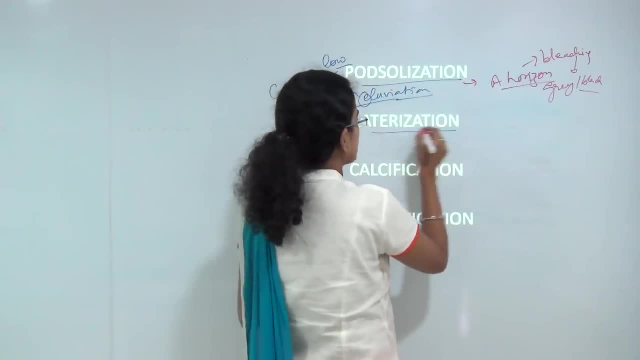 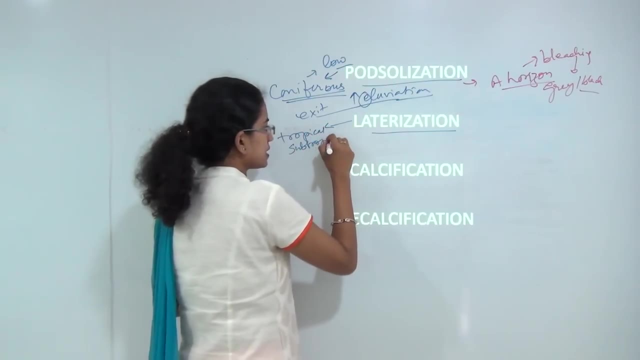 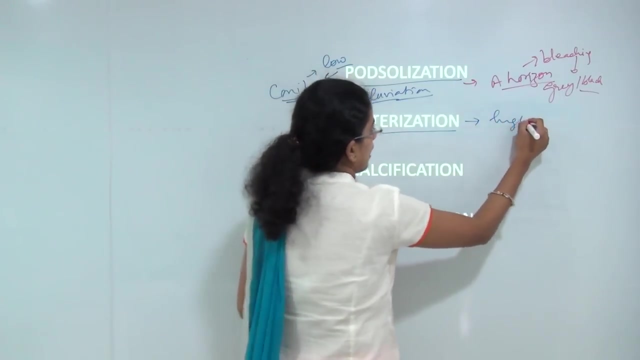 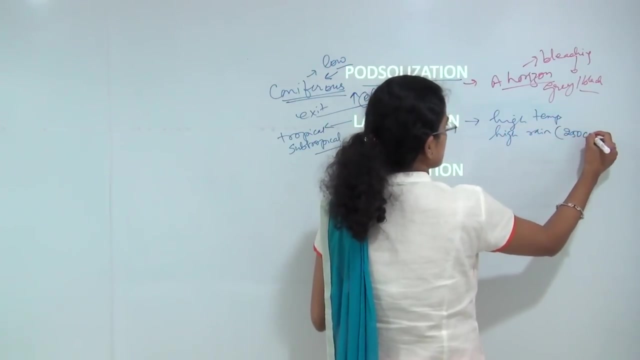 top layer of the soil. In contrast to podocelization, lateralization occurs in tropical and subtropical areas. The region where lateralization occurs is basically a region of high temperature, high rainfall. So you have high temperature, high rainfall, rainfall usually considered greater than 250. 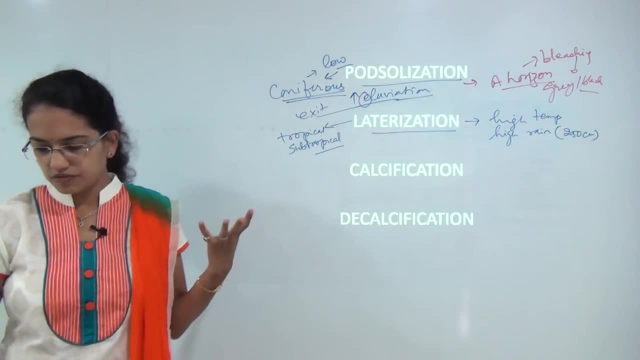 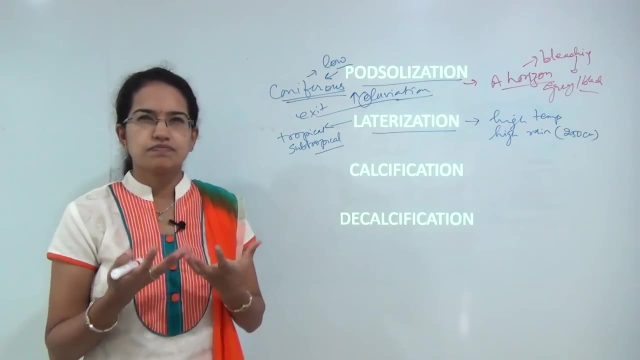 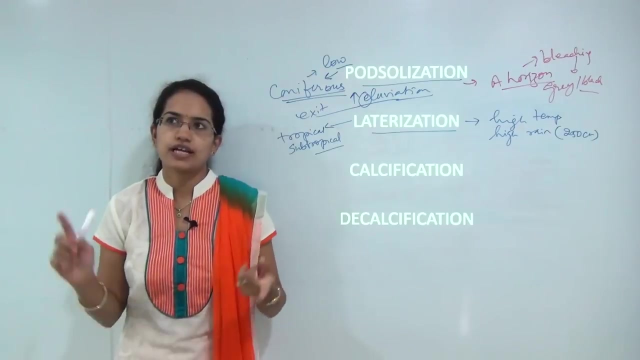 centimeters is the average that we consider for lateralization. Okay, Okay, Okay, Okay Okay. Under lateralization, what happens is you have removal of oxides that takes place and that leaves the caesoxides behind. caesoxides can be in form of either iron or, mainly, aluminum. 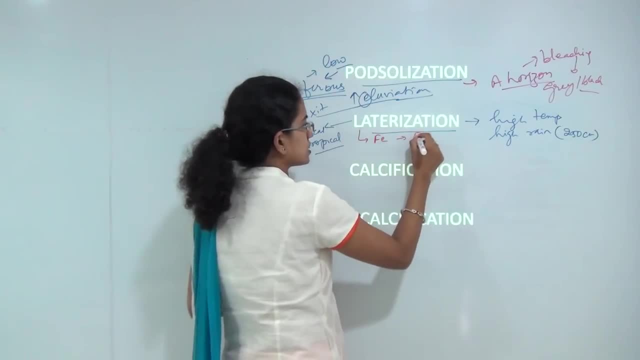 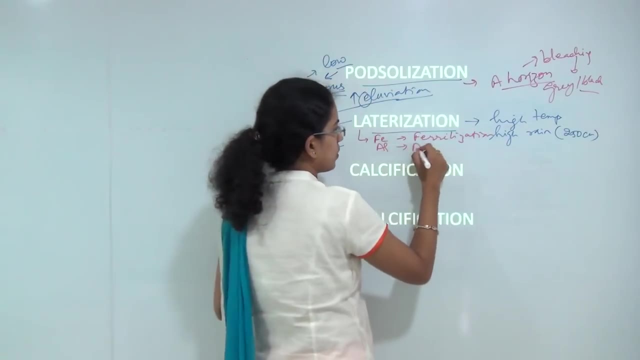 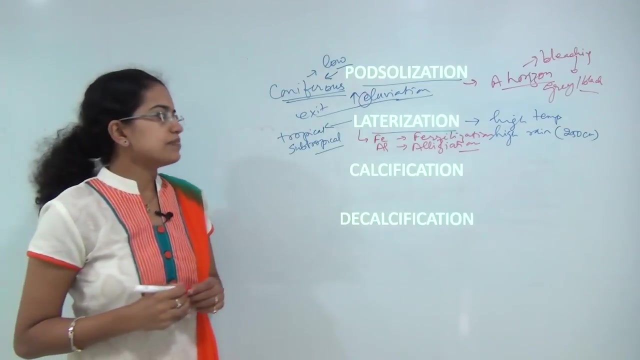 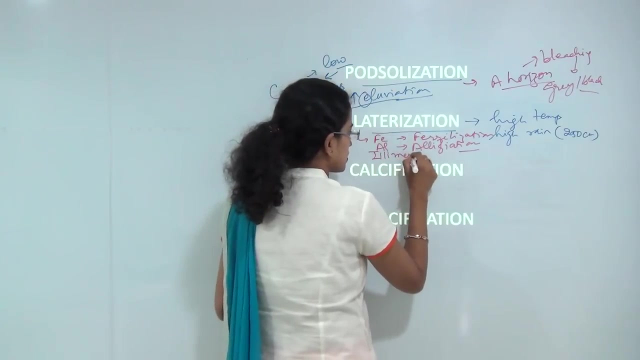 So if it is iron that is left behind, we call this process as feralization. If it is aluminum that is left behind, we call this process as elucidation. Okay, Okay, Okay. And besides this, there is another process, which is known as elimerization, where we talk: 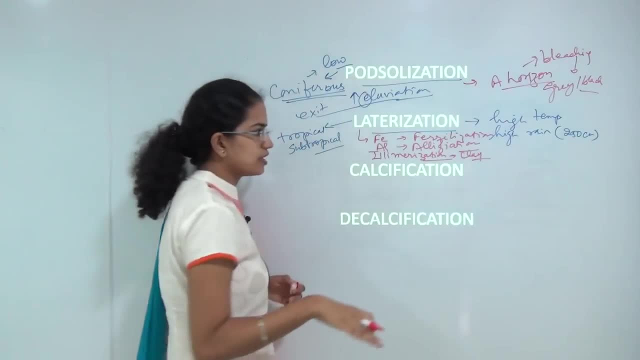 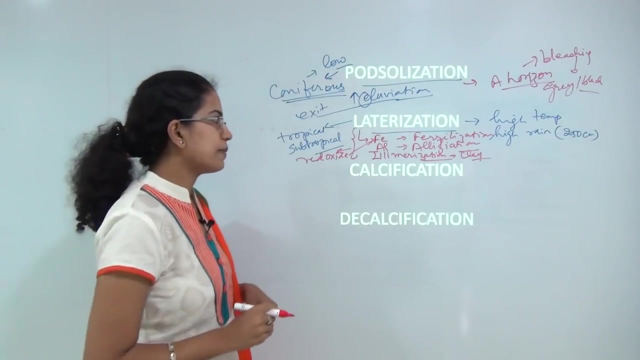 about compaction of clay, or clay moving into the deeper horizons. So that is what is the process of lateralization, and in lateralization you have usually red color or red oxides that are deposited as a result of iron. Okay, Okay, So you have red color layers that are being deposited under lateralization. 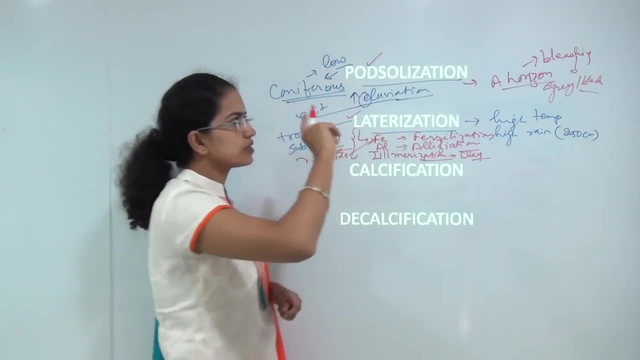 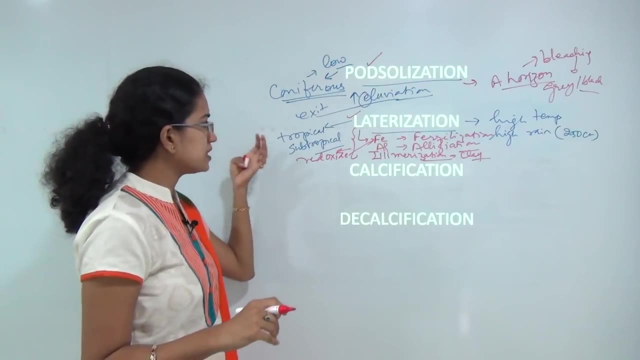 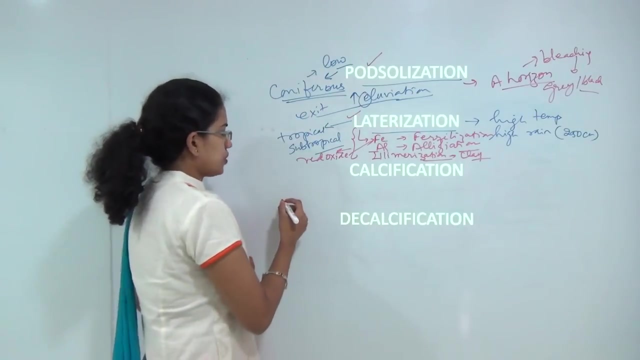 So one of the process that we talked about is podesolization, common in humid, cold mid latitude regions. Then you have lateralization, common in tropical and sub tropical regions. Now let us do calcification and decalcification together. So let us say: I have carbon dioxide plus water. 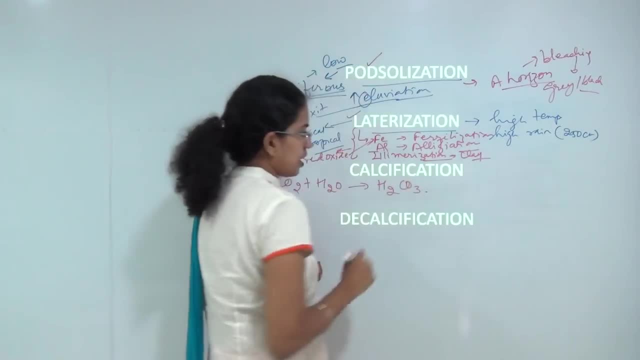 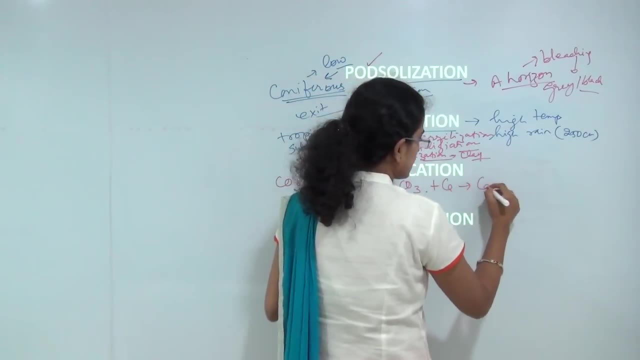 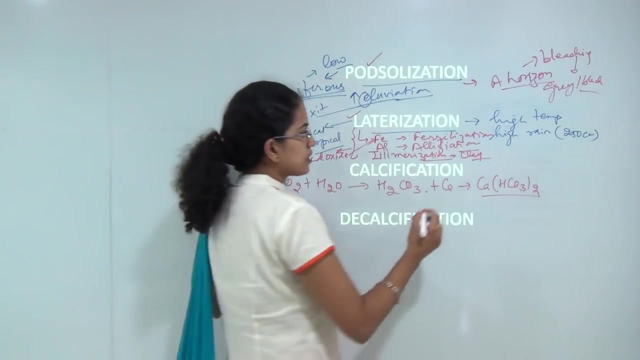 This would give me hydrogen bicarbonate. Okay, Okay, Okay, Okay. So this hydrogen bicarbonate and this H2CO3 when reacts with calcium, I get calcium bicarbonate. Now I have calcium bicarbonate with me. This calcium bicarbonate is soluble in nature. 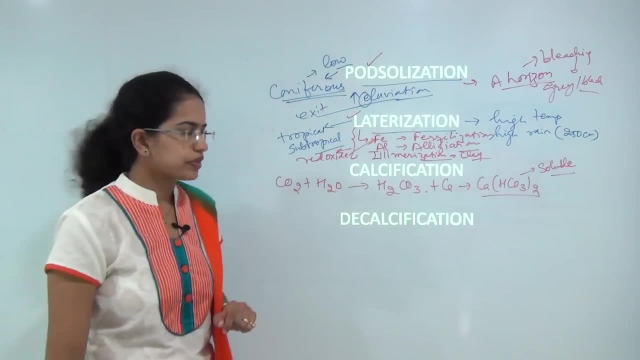 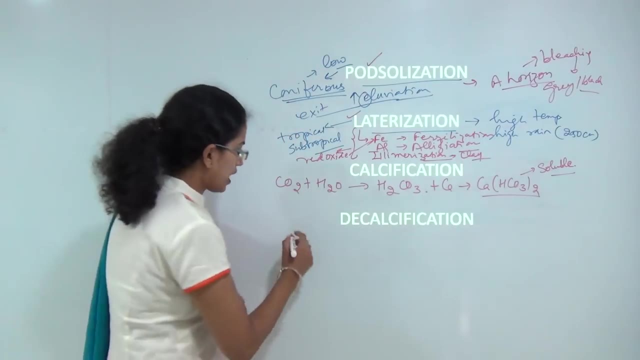 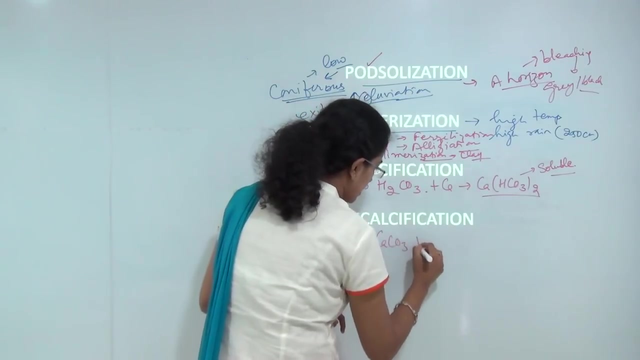 So, since it is soluble, it will percolate down. that is what is happening in the process of decalcification. While in the process of calcification what happens is this calcium bicarbonate that I have- Okay, that I have- breaks down into calcium carbonate, water and carbon dioxide, and this calcium 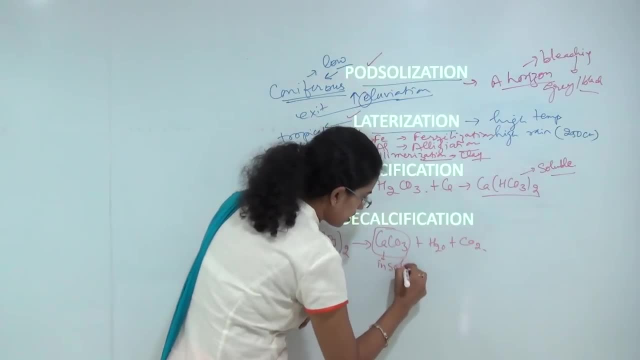 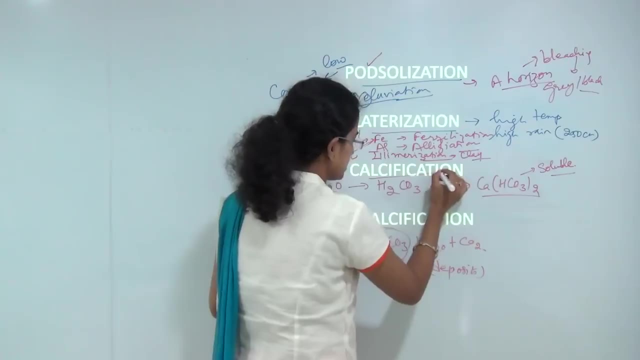 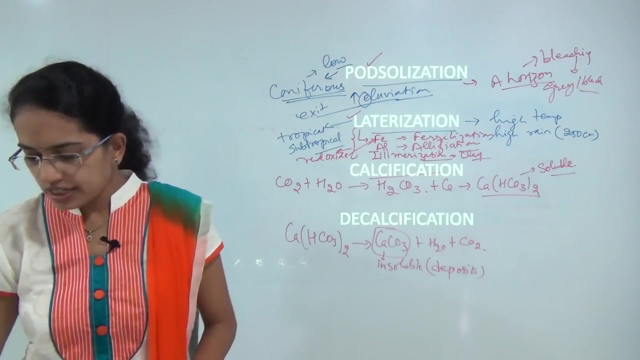 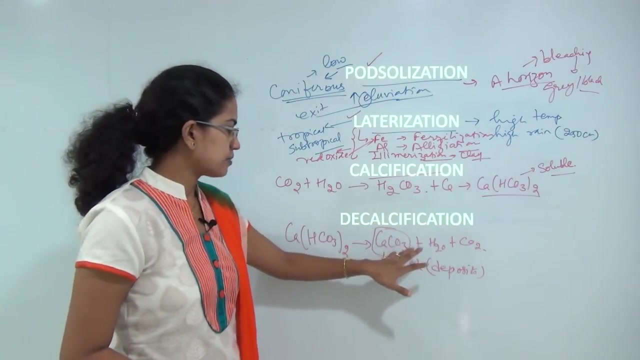 carbonate is insoluble and it kinds of deposits. So what happens under the process of calcification is this: calcium carbonate gets deposited as cations and B horizons usually. in contrast to this, under process of decalcification the leaching of calcium carbonate occurs. and this calcium carbonate, when it is leached down. 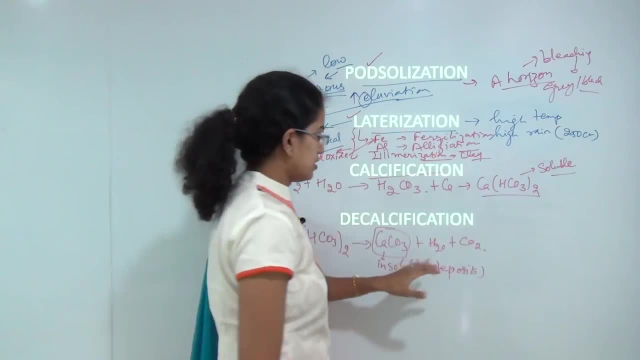 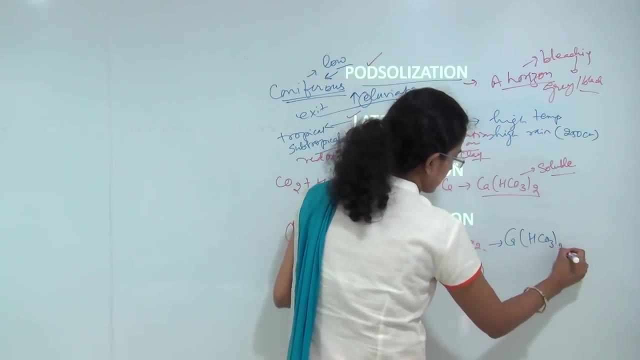 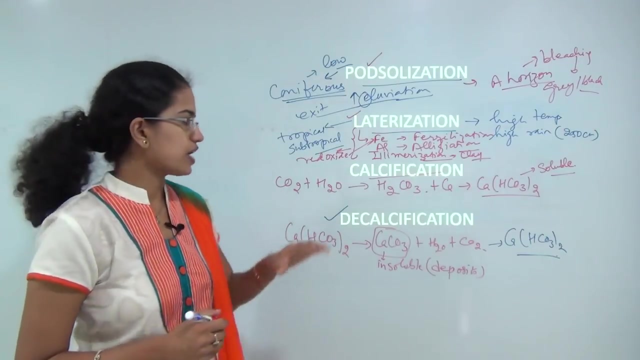 it forms calcium bicarbonate. So when it is leaching, it again combines with water and carbon dioxide and forms calcium bicarbonate, and this, which is soluble, leaches down, and this is what happens in the process of decalcification. So we have the process of calcification, where insoluble calcium carbonate gets accumulated. 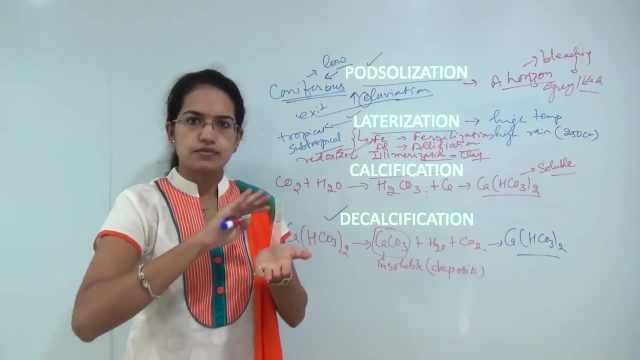 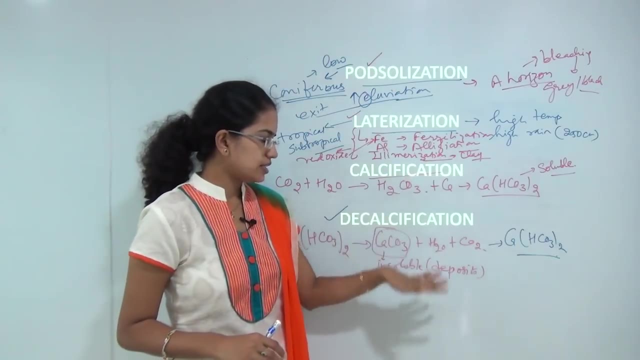 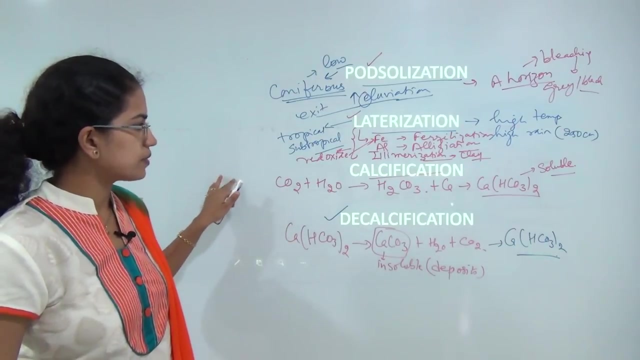 in the top layers in forms of cations and B horizons, while in decalcification, reverse of calcification takes place, that is, leaching of calcium carbonate takes place and it forms calcium bicarbonate, which is soluble in nature. So these are some of the processes of soil formation. 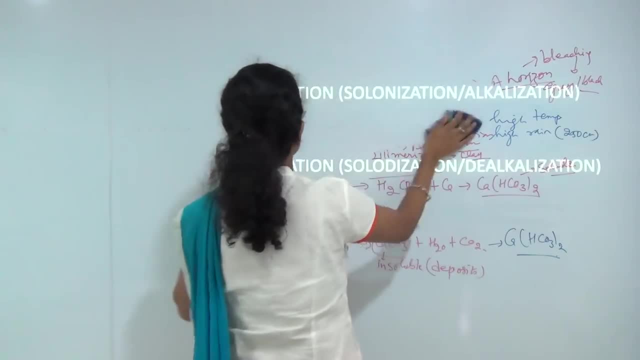 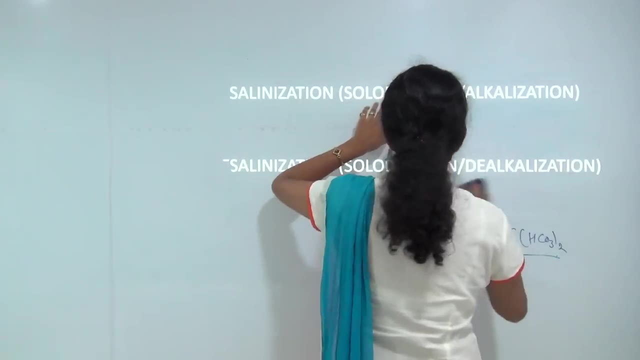 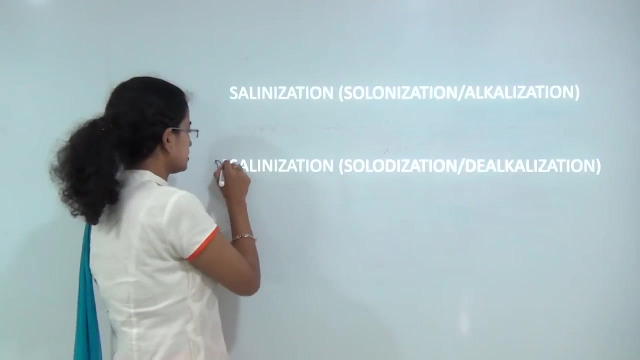 Now let us move on to the next important processes under soil formation. It is known as de-calcification. Now, de-calcification is also known as solonization or alkanization. in contrast to it, de-salinization is known as sodalization, and this is solonization. 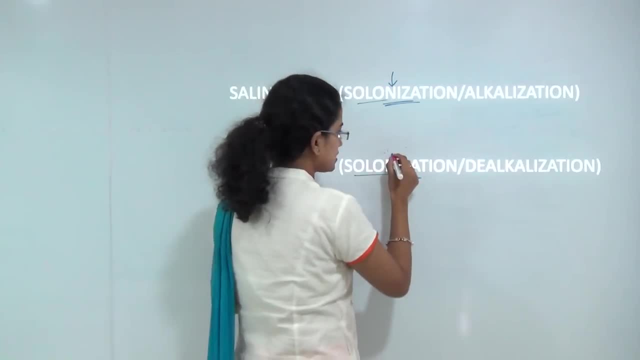 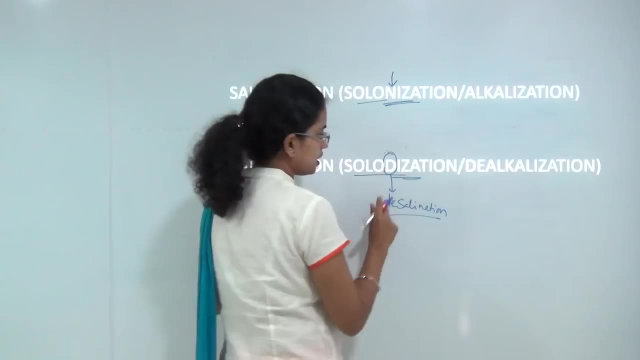 So solonization is salinization and sodalization, since it is d here, it is, stands for de-salinization, So that is the best way to remember: so for d for d. So, rather than getting confused with MCQs and other questions, it is important that we try to remember using some mnemonics. So you have solonization, that is salinization. in contrast to that, sodalization is de-salinization, and this sodalization is also known as de-alkanization. in contrast, salinization is known as alkanization. So what happens under salinization is you have addition of sodium. that takes place while in de-salinization, As the name suggests, d means removal, so there is removal of sodium, So removal of sodium takes place in de-salinization. so, under de-salinization, what is happening? 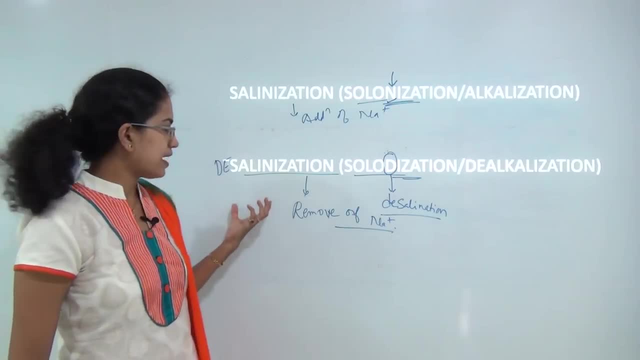 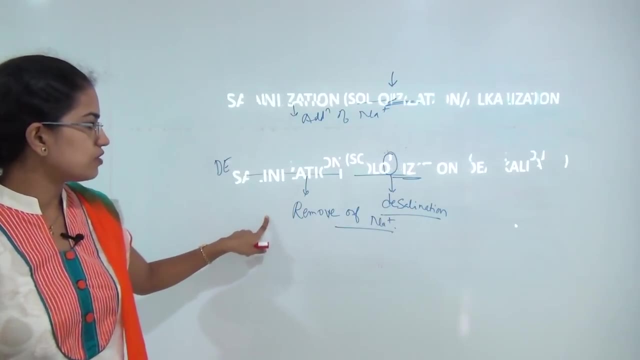 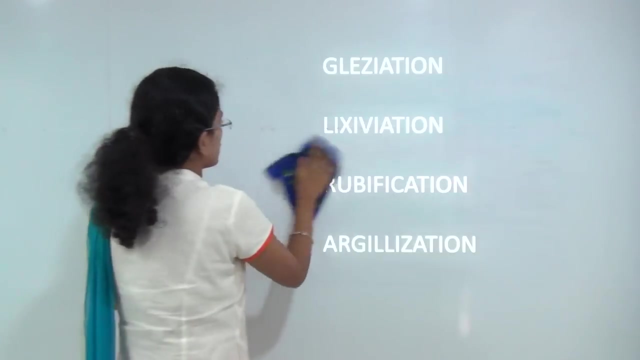 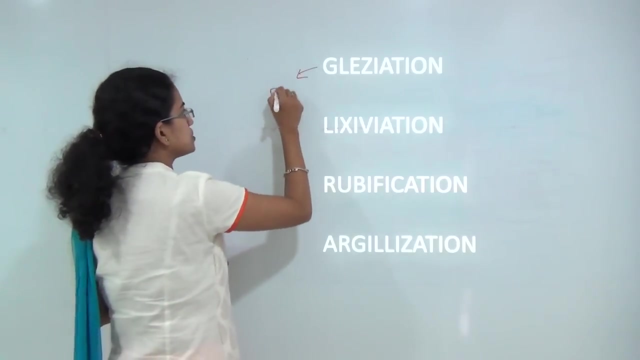 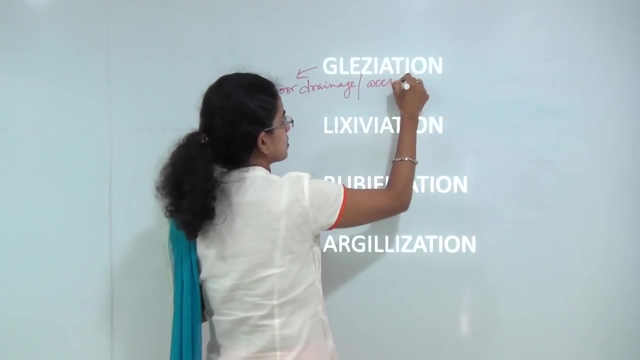 is, you have hydration of sodium ions that is taking place. as a result, there is concentration of calcium and magnesium that is causing this dispersion of sodium ions. The next few terms that we would be discussing today are Glaciation. Now, glaciation is usually formed due to poor drainage or accumulation of organic matter. 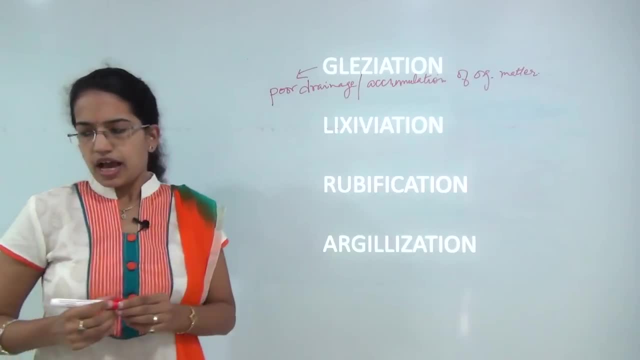 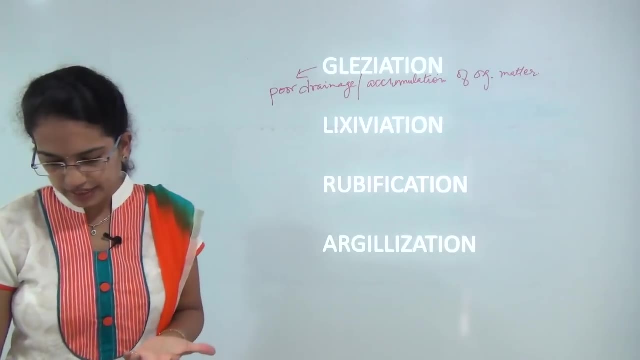 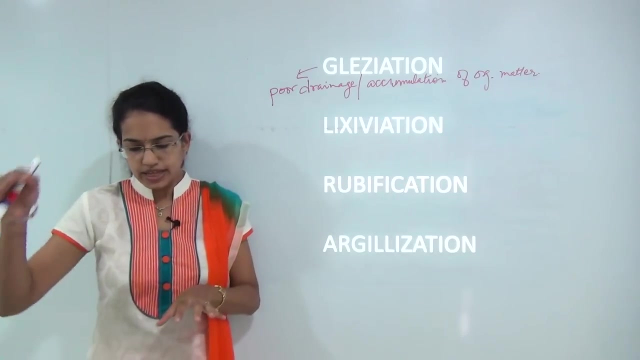 So what happens under glaciation is: iron is converted into soluble iron form, since there is poor drainage and accumulation. So what happens under de-salinization, Glaciation of organic matter? the reduction of iron takes place, So iron comes out into a soluble iron form that goes and leaches down. when it leaches, 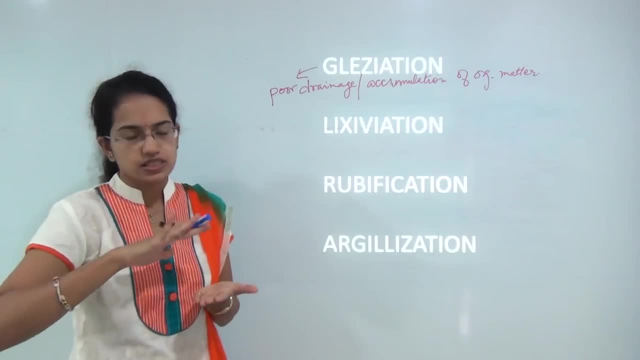 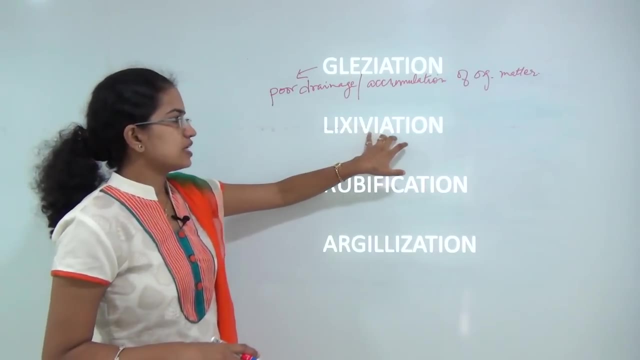 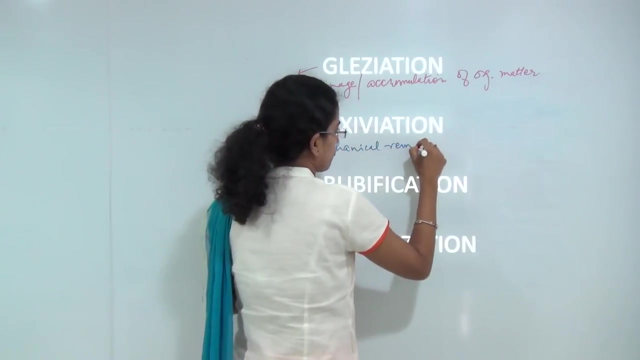 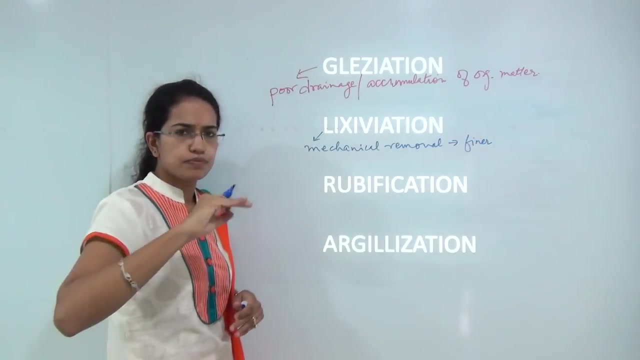 down, there is a kind of surface layer that is glazed and that is known as glaciation. The next is lexiviation. under lexiviation you have mechanical removal of finer particles, Glaciation, Glaciation, Glaciation From the soil, so you have that soil, and from the top layer of the soil you are mechanically 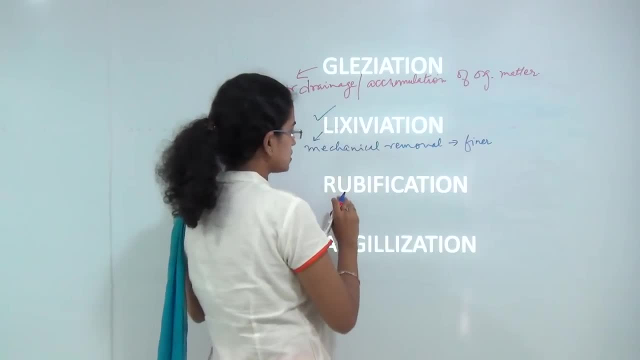 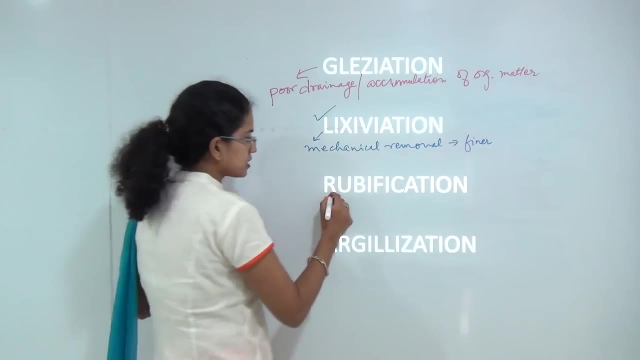 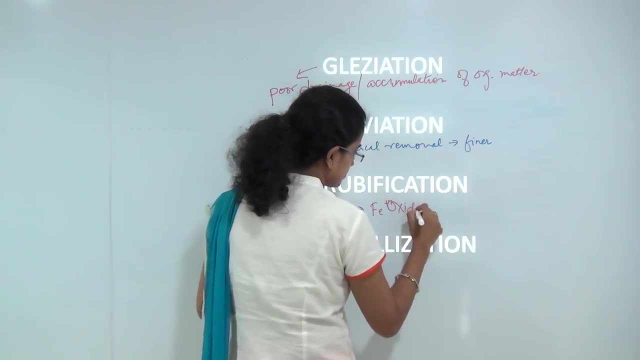 removing material, so that is known as lexiviation. The next is rubification. what happens under rubification is iron is released to form free oxide. so you have iron that is released to form free oxide. Glaciation, Glaciation, Glaciation. 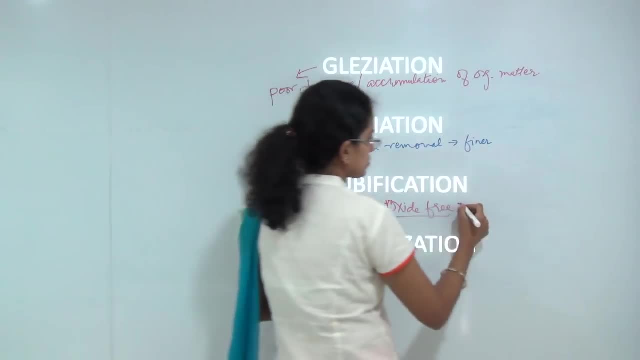 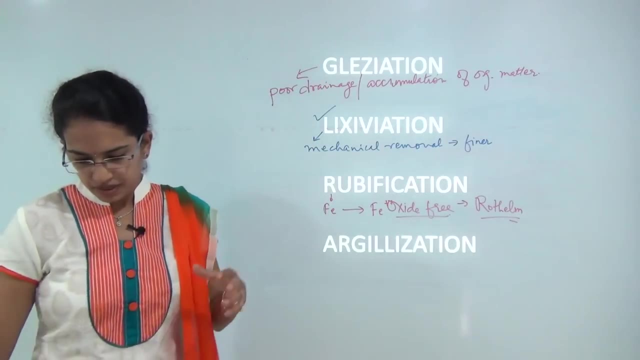 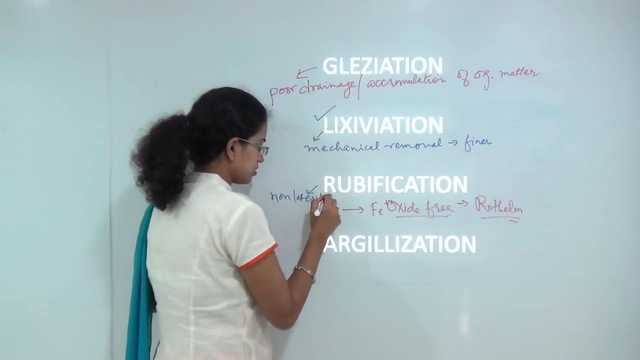 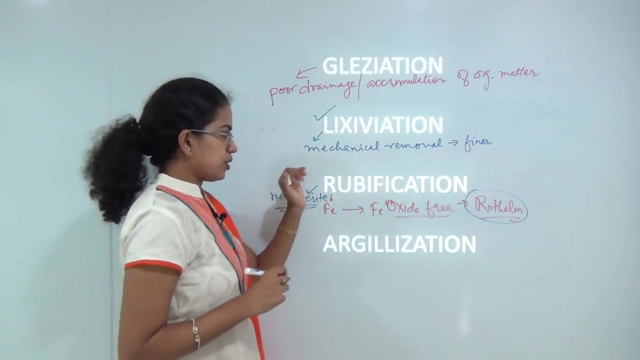 Glaciation, Glaciation Here. rubification is known as Rothilum, and this iron, which is released as free oxide, forms a non-laterite coating over the surface, and this non-laterite coating, which is later on known as Rothilum, is established under the process of rubification. 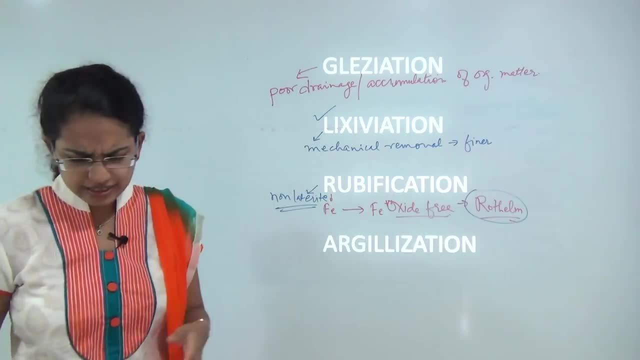 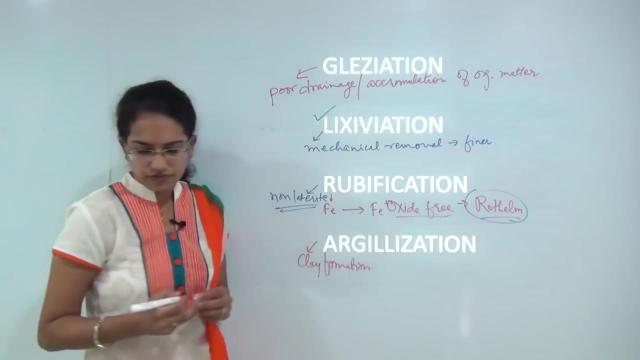 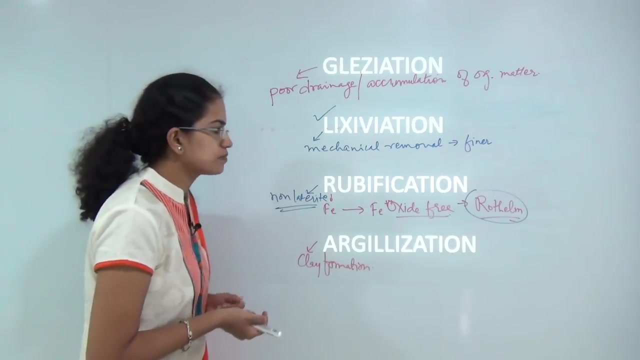 The last is ergalization. under ergalization, clay formation takes place. So you have under the process of ergalization, you have clay formation that takes place due to any chemical composition or chemical change that is taking place. So these were some of the specific processes that we have talked about dealing with soil.